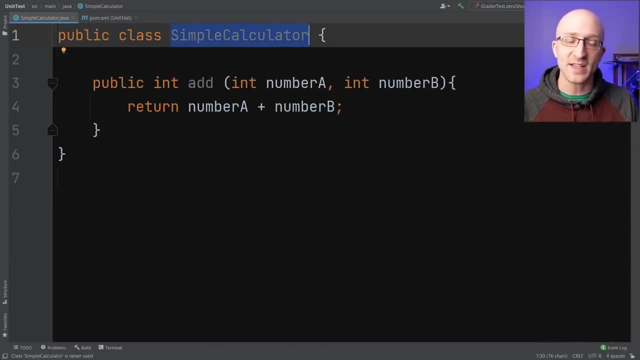 for. So here I have a class called SimpleCalculator, and all it has is a single method called add that just takes in two ints, number A and number B, and adds them together and returns the sum First. how do we even go about creating a unit test If you're using IntelliJ? 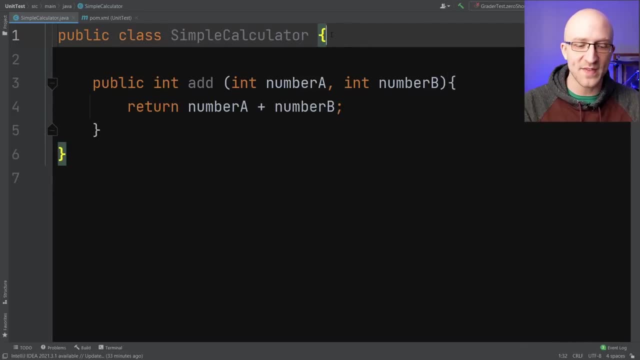 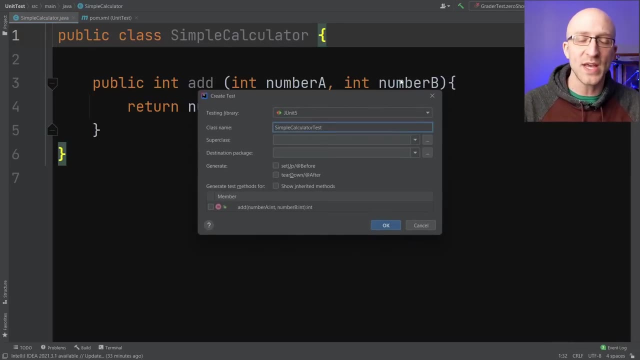 there's a shortcut. All you have to do is have your cursor somewhere inside the class that you want to create a test for and hit control shift T. That'll give you a little pop-up and you can just click create new test. It's automatically using a certain pattern for the test class names. 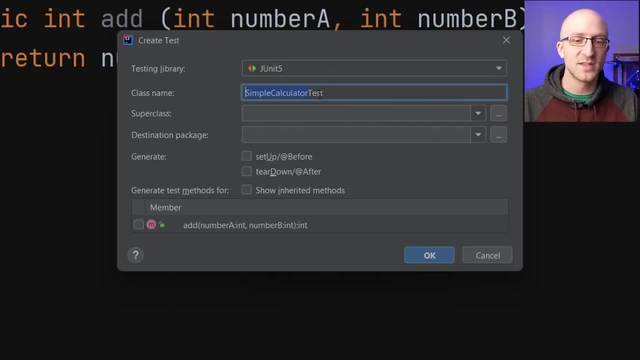 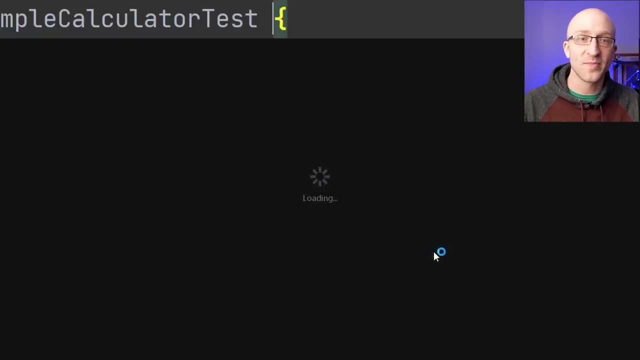 that it creates. Since this will be testing the SimpleCalculator class, it names the test file SimpleCalculator test, And that's totally fine. That works for us, So let's go ahead and click OK. What that will do is automatically create a test class for you. You can see at the 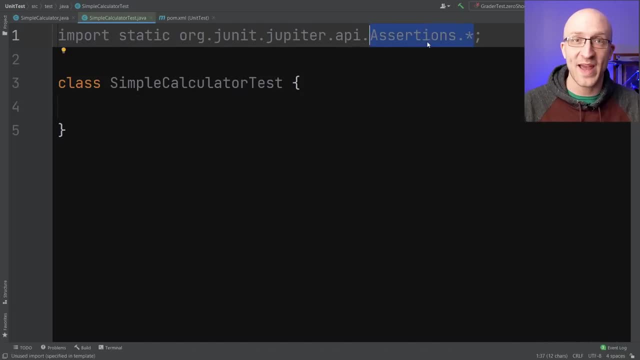 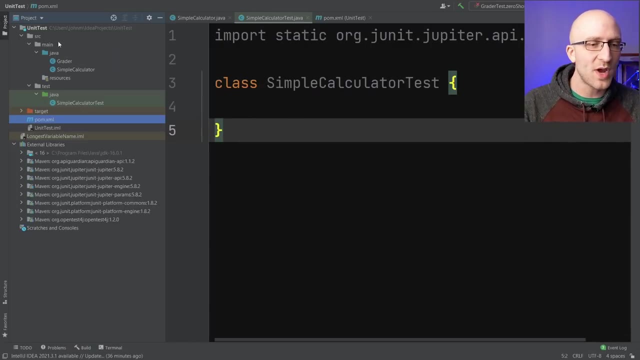 top here that it automatically imported everything in this assertions package, and we'll talk more about that later. Also, it's important to note exactly where it created this test file. So if you go over into your project view, we can see that our SimpleCalculator class is under source. 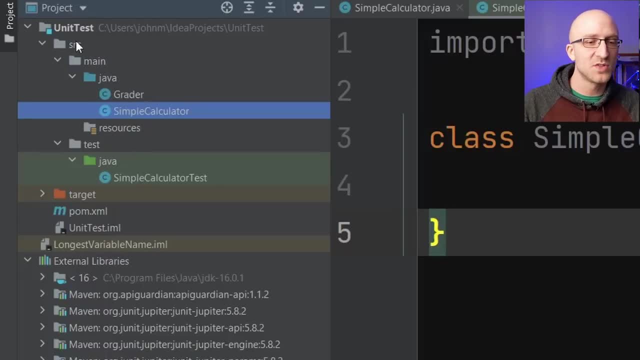 main Java and the unit test file that it created is under source test Java, And that's exactly the convention that you'll see. Any test that you create is going to be in the exact same package structure as the file that you're testing. only it'll be under source test instead of source. 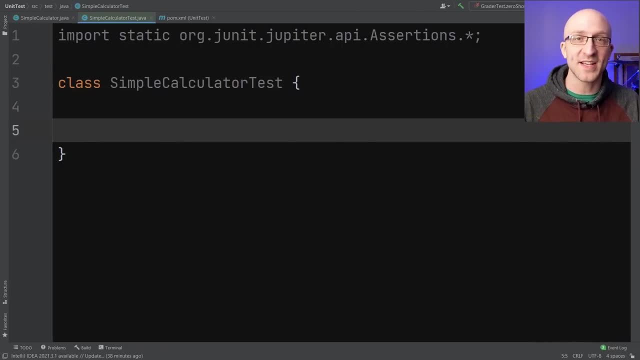 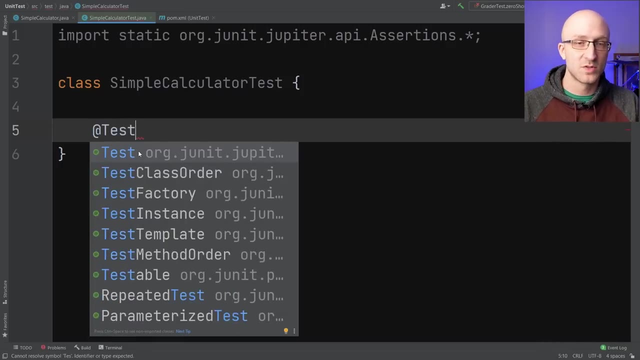 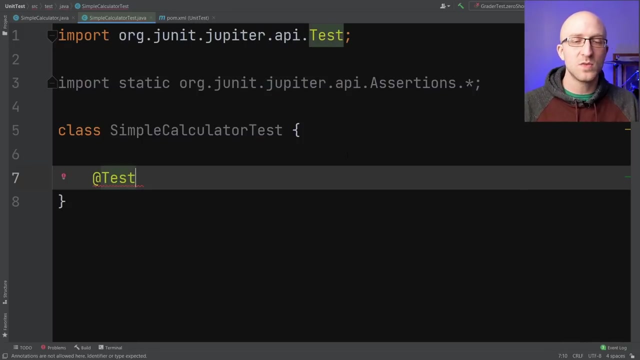 main. Okay, so let's go and write our first unit test In JUnit. a unit test is just a method that you label with the at test annotation. So just type in at test and this is the dependency you want: orgjunitjupiterapitest. So now we have to decide what exactly we want. our first unit test. 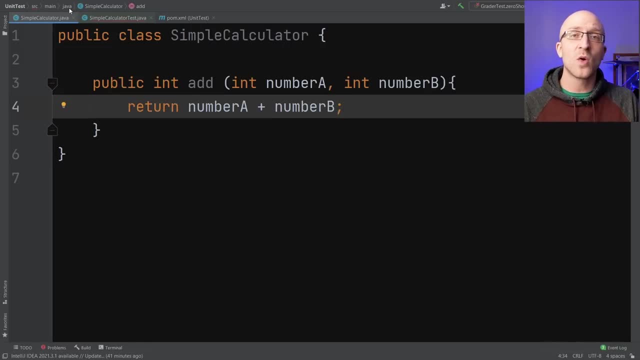 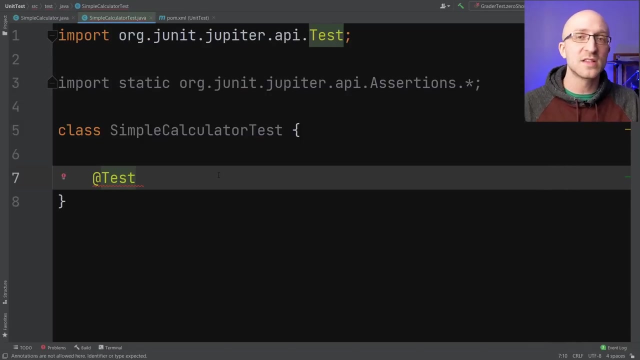 to be. In general, you want to make sure that you have a unit test that's going to be in the name of your test file, So let's go over here and write our method to do that. As long as you're using JUnit 5, your test methods don't need to be public and they don't need to return anything. So 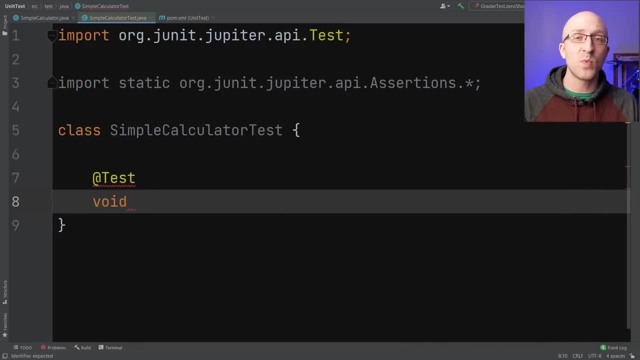 your return type is just going to be void. Next, you want to come up with the name of your test, and it can be whatever you want. It's just the name of your test method, But it should be something that's very descriptive of the exact scenario being tested here and what. 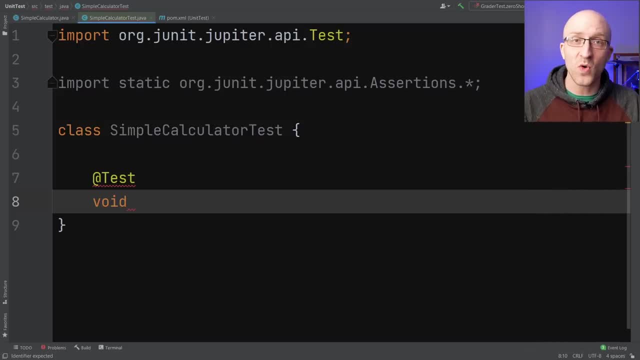 the result should be Here: we're just testing that 2 plus 2 should equal 4.. So let's make that our method name: 2 plus 2 should equal 4.. This method won't take any parameters, so we can just. 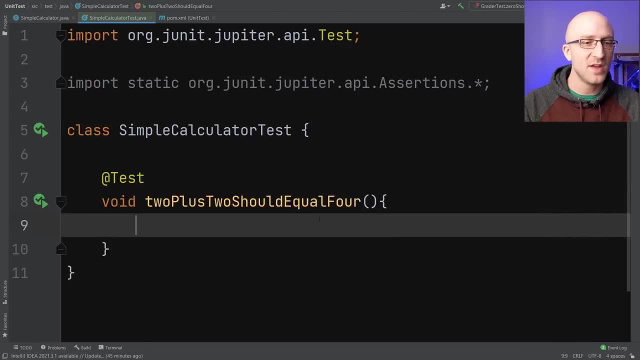 have an open and close parentheses here Inside this test method. we want to call this simple calculator's add method. So first let's go ahead and create a simple calculator object that we can actually call this method on. So simple calculator- calculator equals new, simple calculator As a 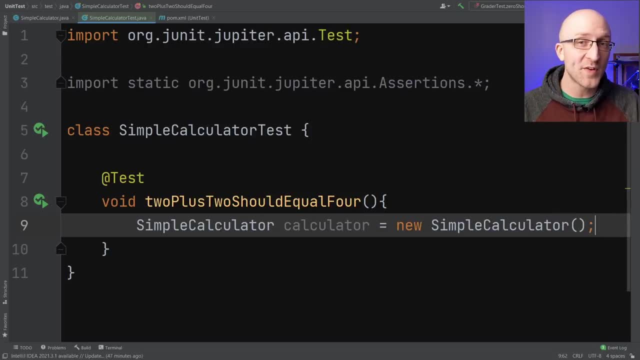 quick tip: ever since version 10,, Java has what's called local variable type inference, which basically means that when you're creating a local variable like this, instead of using the entire class name here, Java can infer what the type of this variable is supposed to be. So you can. 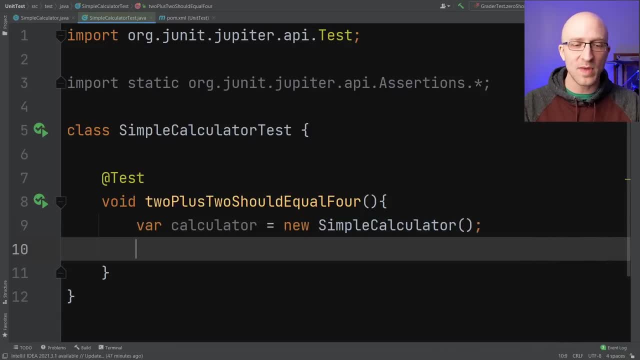 actually just put var here. So now we want to call the add method on this calculator object, So calculator dot add, And we want to test adding 2 plus 2.. So we'll send in 2 and 2.. This add method is going to return a. 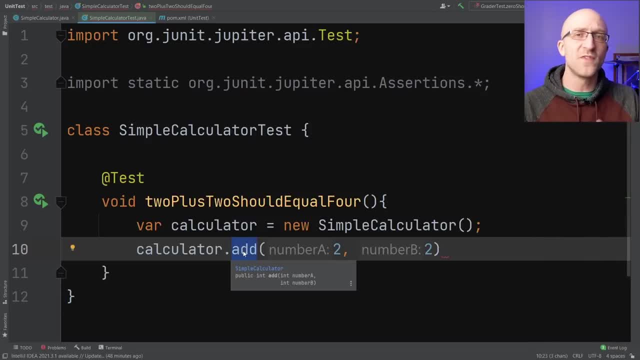 result, And here we want to verify that it's returning 4.. So how do we do that? In JUnit and in pretty much every unit testing framework, when you want to do that type of verification, you use what's called an assert statement. So here we want to verify, we want to assert that the result 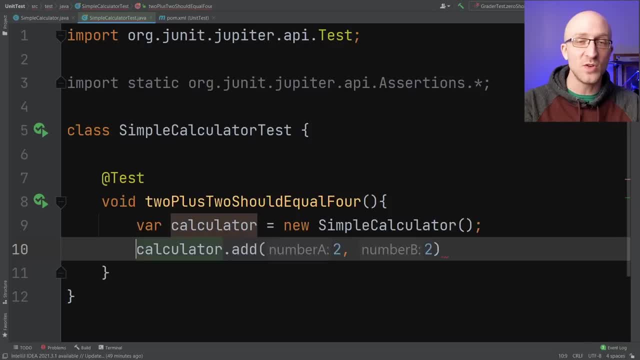 of this method call equals 4.. To do that we can use a method built into JUnit called assert equals, And that method gets two parameters passed into it. The first parameter is the value that you expect the result should be. So we expect that 2 plus 2 should equal 4.. 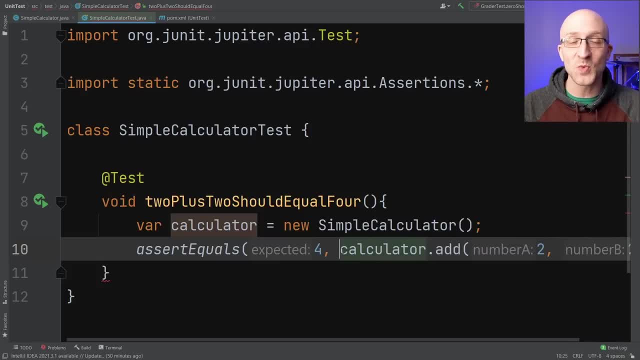 The second parameter that you pass into assert equals is the actual result of your test. So the actual result of our test will be whatever calculator dot add returns when we send in 2 plus 2.. So let's just close our parentheses and add a semicolon, So we're saying that the result 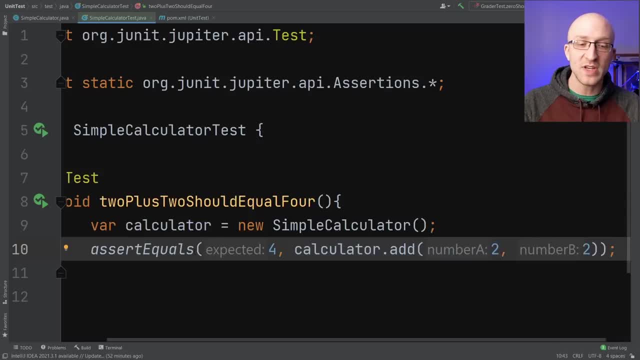 of calling this add method is going to be 4.. So we're going to pass into assert equals And that add method with 2 and 2 should equal 4.. And if it doesn't, our test will fail. So now we have our. 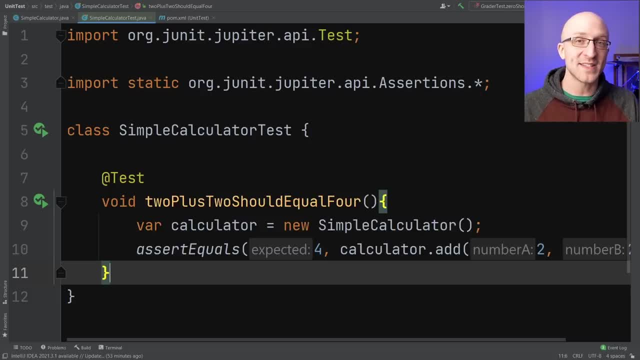 first unit test. How do we run it and make sure that it passes In IntelliJ? there's a couple of ways. Probably the simplest is next to each test method. you'll see this icon here in the margin. This allows you to run that particular test And when you click it it'll give you a couple of 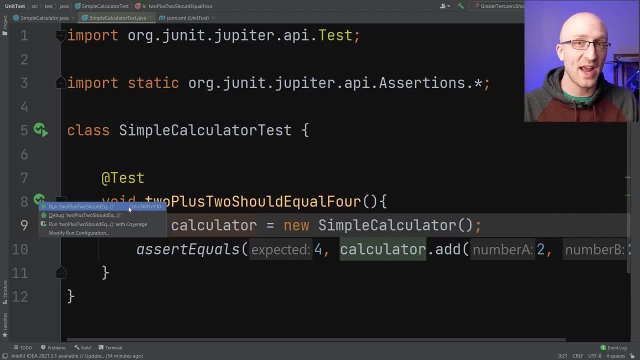 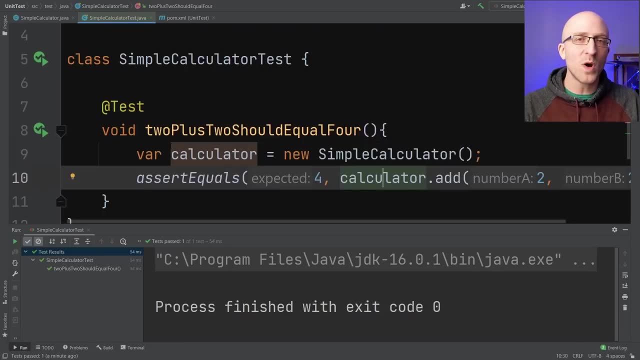 options. This first option will just run your test. So let's go ahead and click it and see what we get. All right, so it's telling us all of our tests passed. So this test seems to be working great. But what would we have seen if? 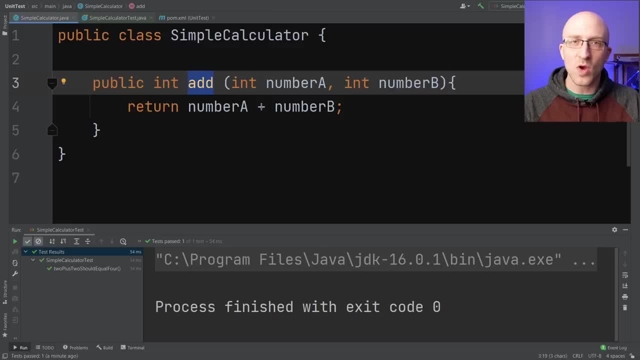 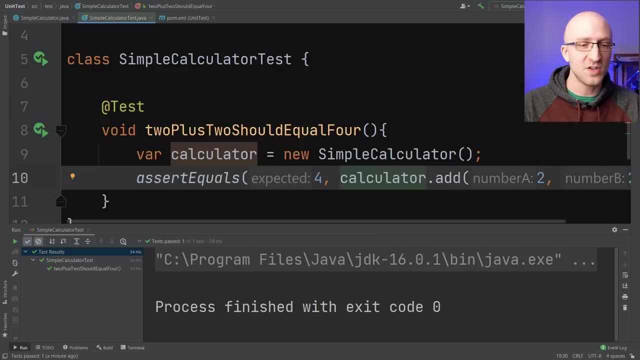 this test failed. So what if our code was doing the wrong thing And instead of adding these two numbers, it was subtracting them? So now, because the code isn't doing the right thing, our test should fail. So let's go ahead and run it again. Okay, so now we see that our test failed. And if 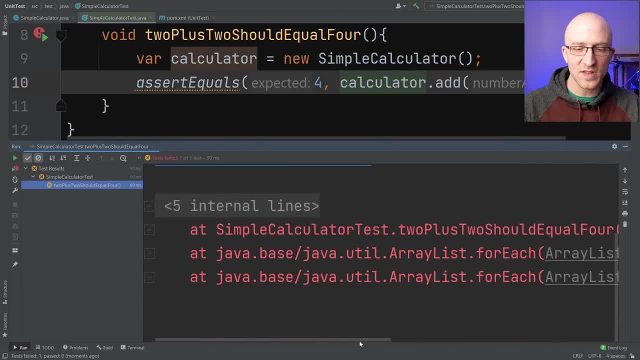 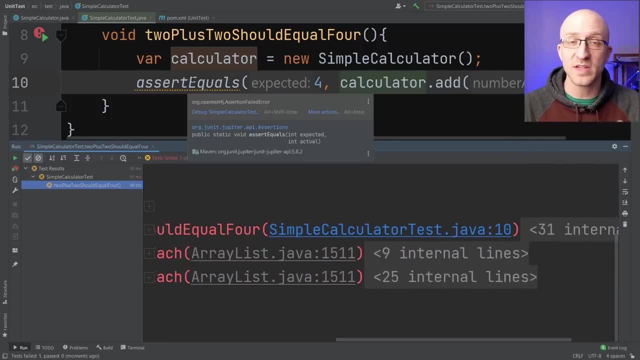 we click the result of that test. it shows us exactly the line in which that failure happened, which is simple calculator test, line 10, right here our assert equals statement, And it also tells us exactly what the problem with the assertion was. 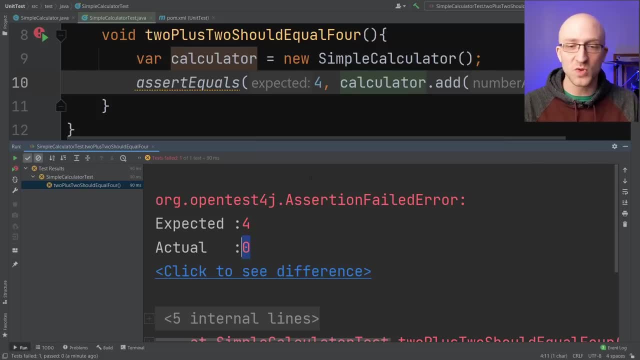 it's telling us that the expected result was four, but the actual result it received was zero. So this assert equals statement fails, failing our test, And in this case that's good. our test should be failing if our code is doing the wrong thing. So if we change this back to addition and rerun our 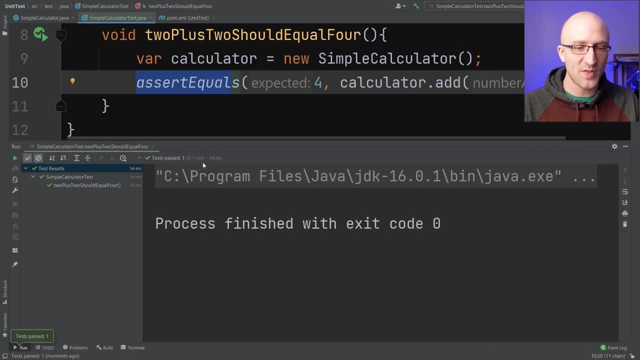 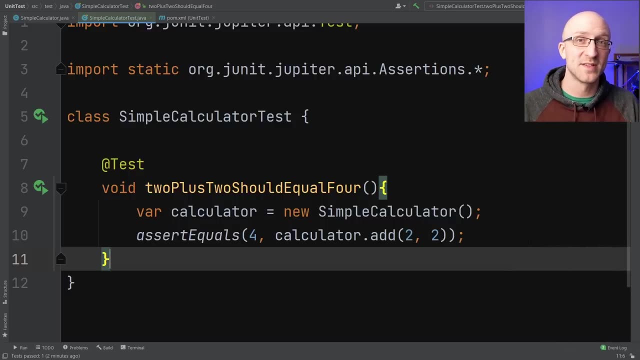 test. we should see it pass again And we do everything passed. everything's green, all good. Virtually all the unit tests that you write are going to have one or more assert statements And there are a lot of different types of them that assert different things. Assert equals is the one. 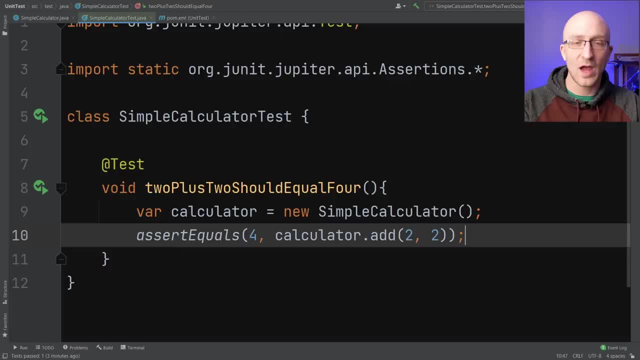 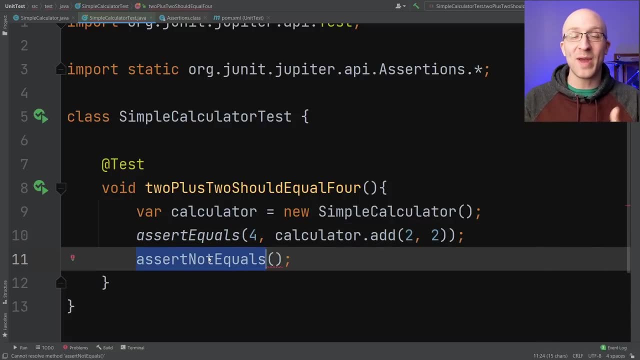 we've already used. that's probably one you're going to be using pretty often. However, if you want, you can also call assert not equals. So with assert not equals, your test will only pass if the two parameters that you pass into that method don't equal each other. And if they do, 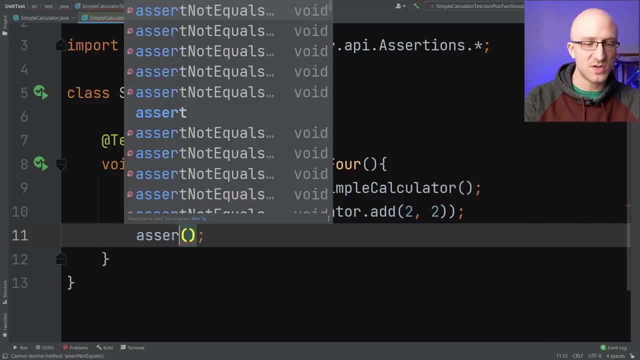 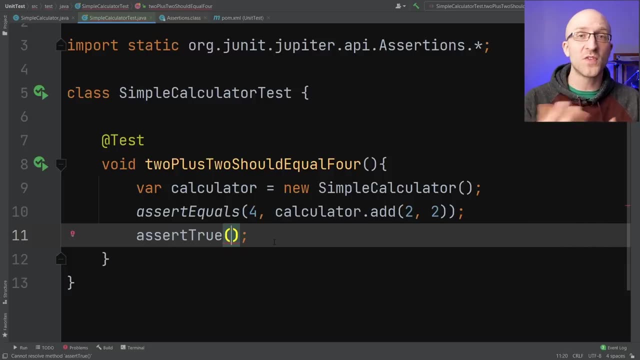 equal each other, your test will fail. You also have assert true, And that will just take in as a parameter some kind of expression that evaluates to a boolean true or false. If that expression evaluates to true, your test passes, And if it evaluates to false, your test fails. 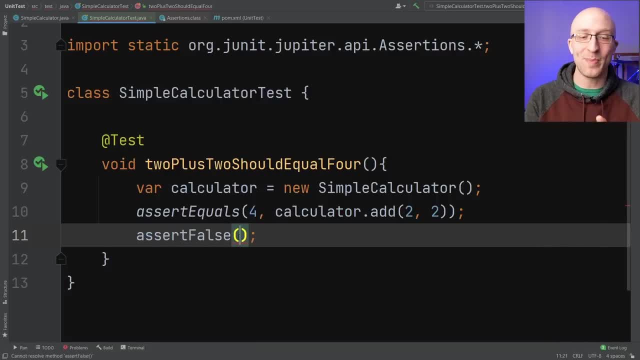 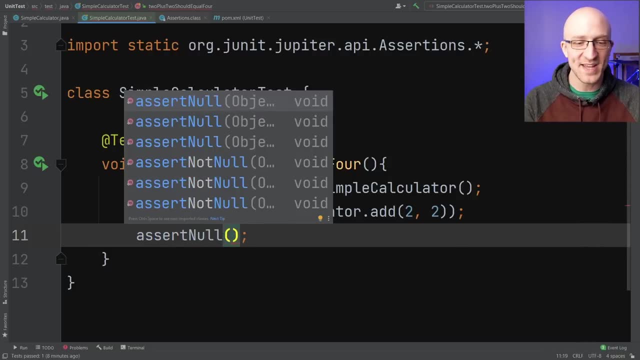 You can also use assert false, which will do the opposite. It'll pass the test when the expression that you send in evaluates to false. You also have assert null, which will only pass the test if the expression that you pass in is null, And you have assert not null, which will only pass. 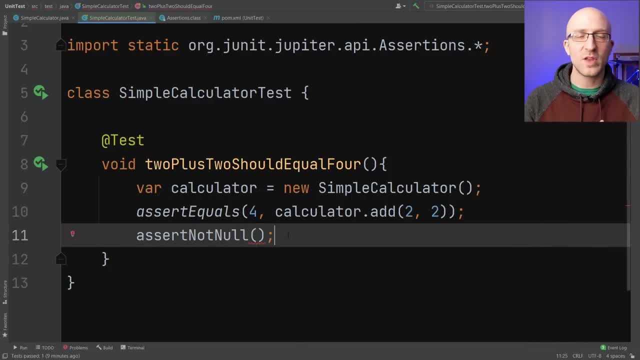 the test. if the expression that you pass in is false And you have assert, not null, which will is not null. Now you might be thinking: well, there's a whole bunch of different ways we could use these assert methods to prove that this method is doing the right thing, right? So here we just. 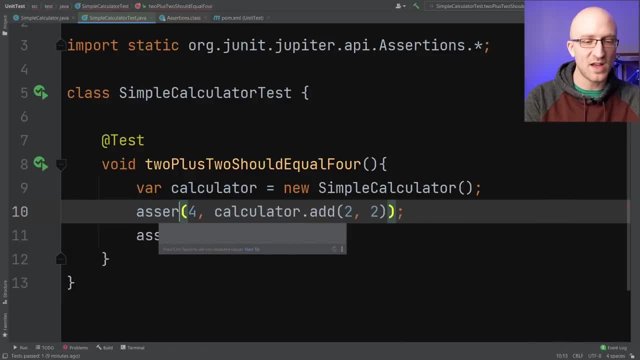 happen to be using assert equals. but we could just as easily have said: you know, assert true, and then we could pass into this assert true method the result of calling this method with two and two double equals four. So using assert true like this is totally valid and will work. 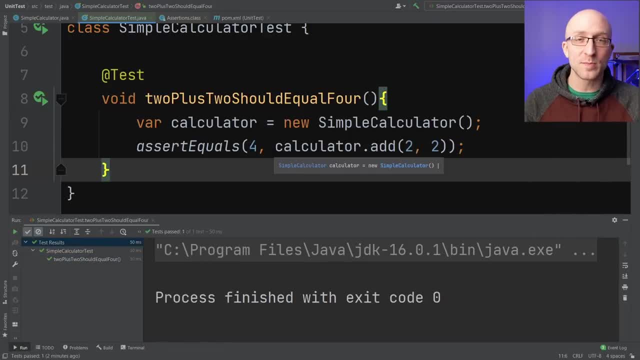 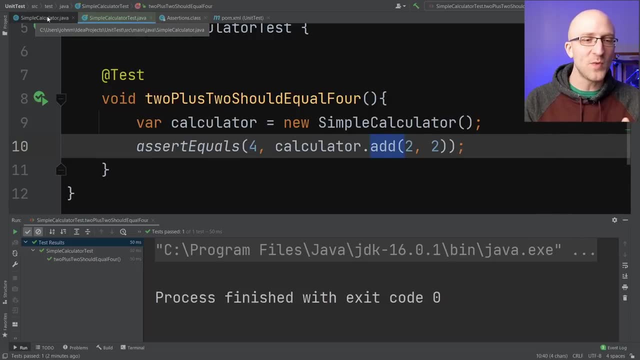 fine, We can see that everything is still passing. There are potentially some problems with just having one single unit test scenario, even for a method as simple as this one. For example, if we go back into our simple calculator and mess up our code in some way. Let's say, instead of doing, 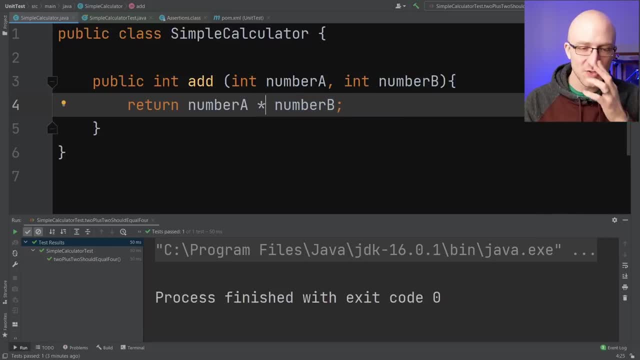 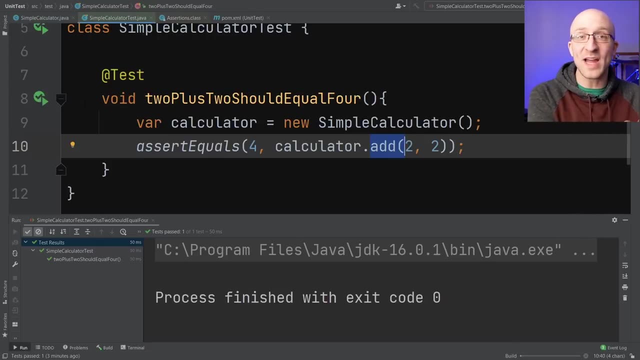 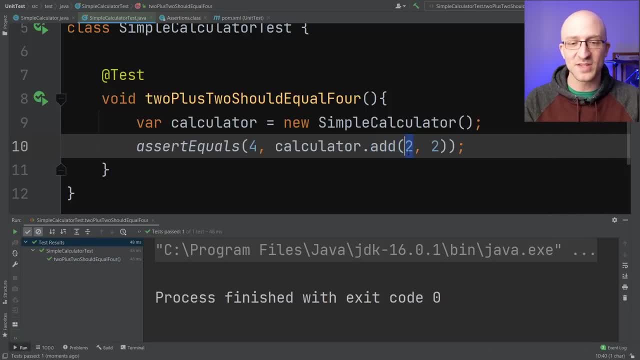 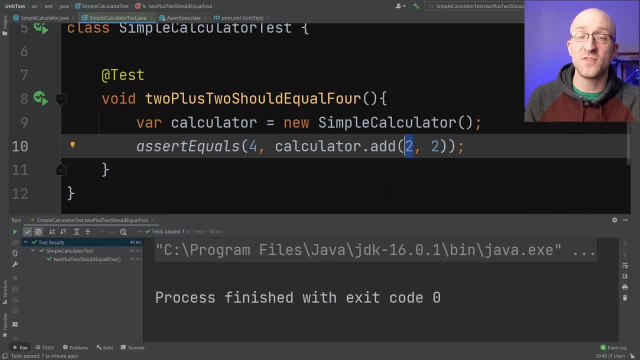 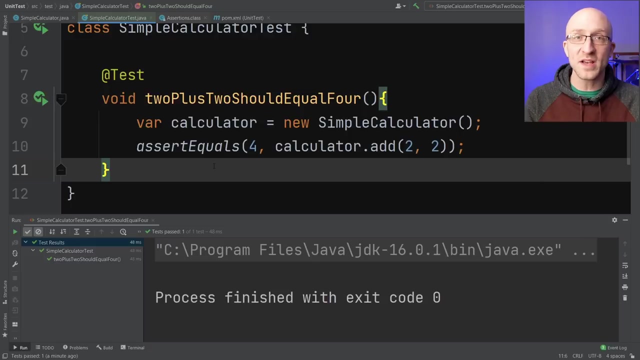 right thing. at least one of our unit tests should fail. Right now, our code is bad. It's doing multiplication instead of addition, but we don't have any unit tests that are failing. Our unit tests are saying everything's great, So that doesn't mean that this unit test is bad. This is a 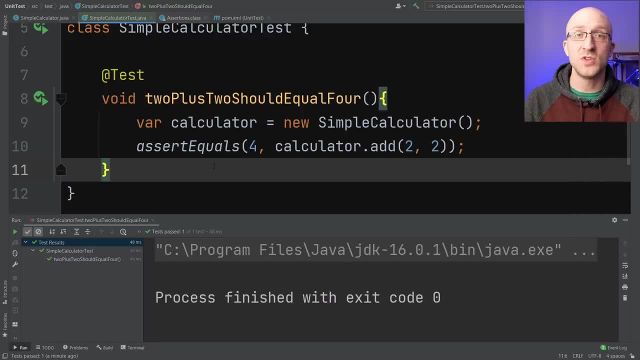 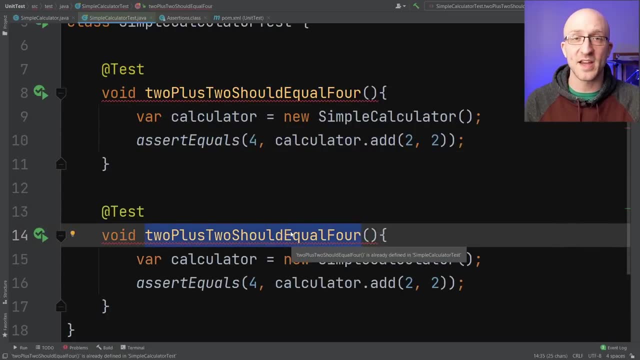 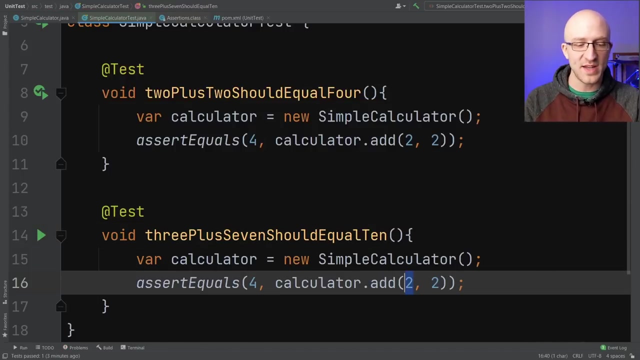 good idea to add more scenarios to our unit test suite. So what you can do is just copy that test method that we made and change it to verify another test scenario. So let's say it was something like three plus seven should equal ten. We'll send in the values three and seven and the value that we 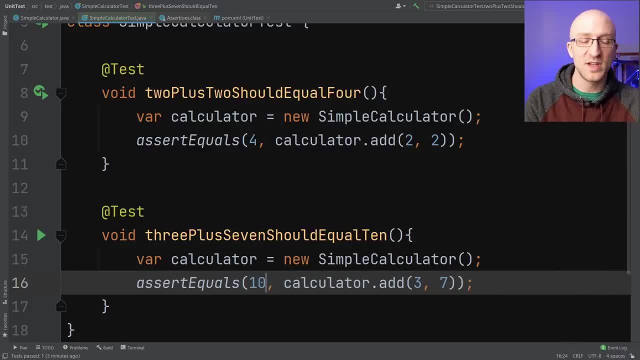 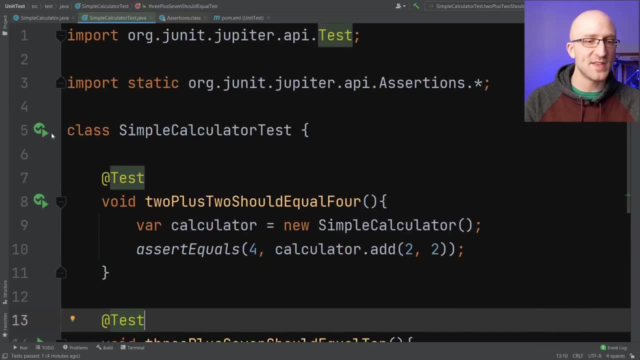 expect when we call this method with three and seven is, of course, ten. Now we could just run this new single test that we just wrote. but we can also just run this new single test that we just have it run all the tests in this class by going up to the class declaration in the margin here. 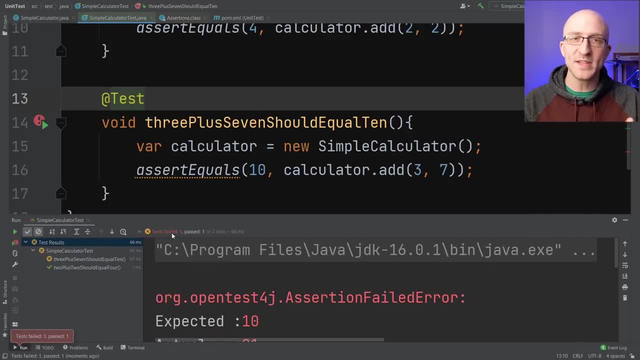 and clicking this to run all tests. All right, so it's telling us one test failed and one test passed. Of course, as we saw before, our two plus two should equal four. test is still passing, but now we have a failing test as well, which we should because our code's bad, It's telling us. hey, we 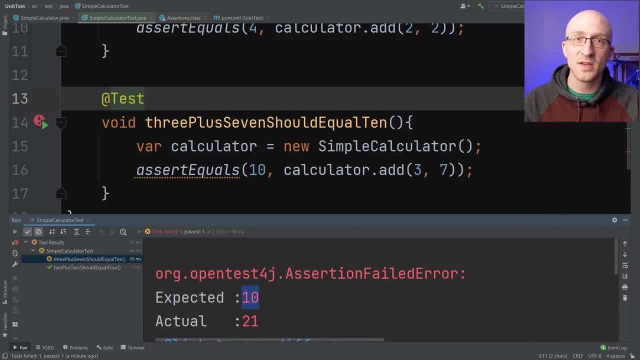 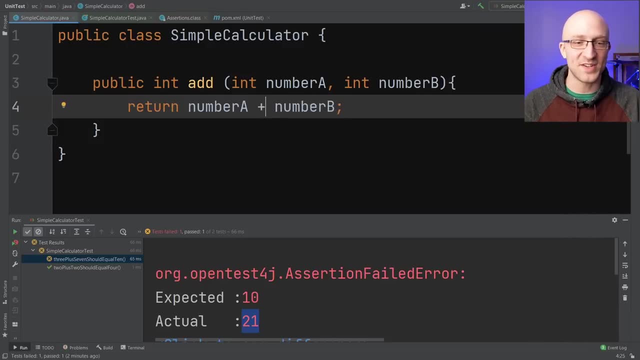 expected this value of 10, but I got the value 21.. So you hop over to this add method in your calculator class and see: ah, some doofus changed the value of ten. Now we can see that we have changed this to multiplication instead of addition. Let's go ahead and click this first. 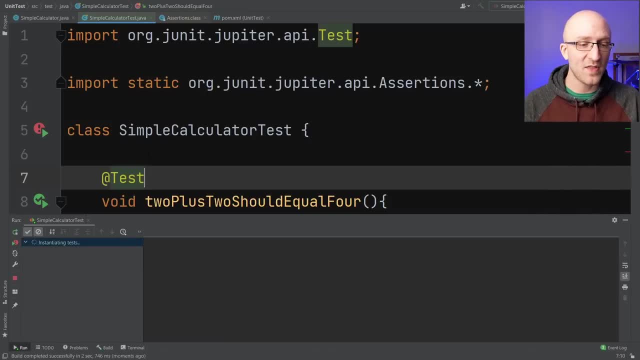 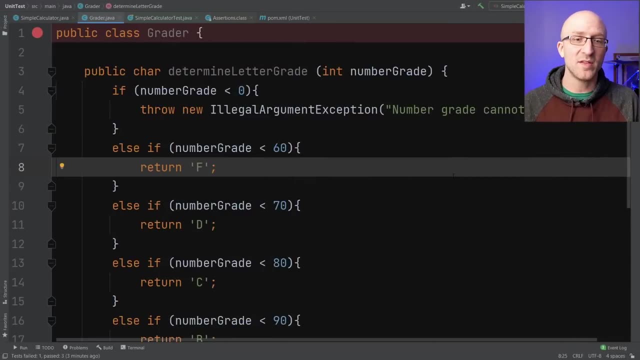 one to rerun all of our tests and make sure our code is good and they all pass. And they do, we're looking good. Now let's try and create some unit tests for a little bit more complicated of a method. This method is called determine letter grade and all it does is take in the number grade. 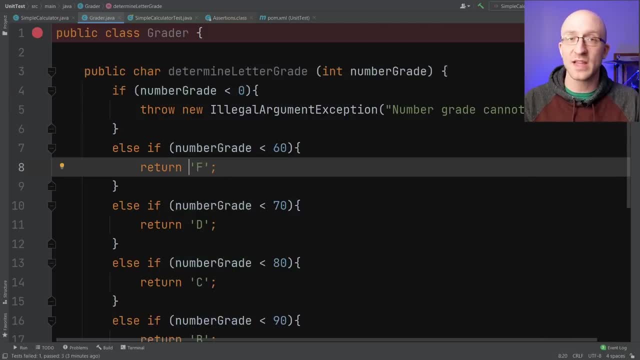 you know the percentage, generally zero to a hundred, and then it returns the letter grade as a character that matches that number. First, anything less than zero is negative and just isn't really valid number grade. so we throw an illegal argument. exception in that case: If it's less than 60, we. 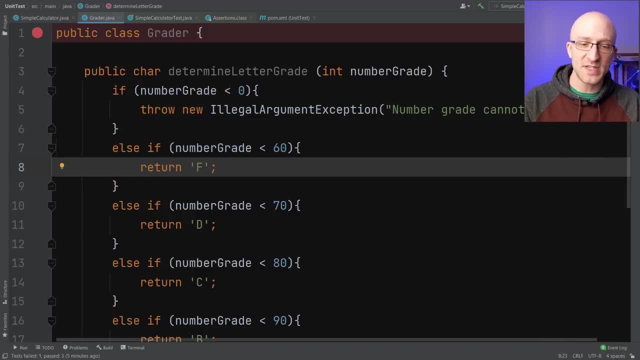 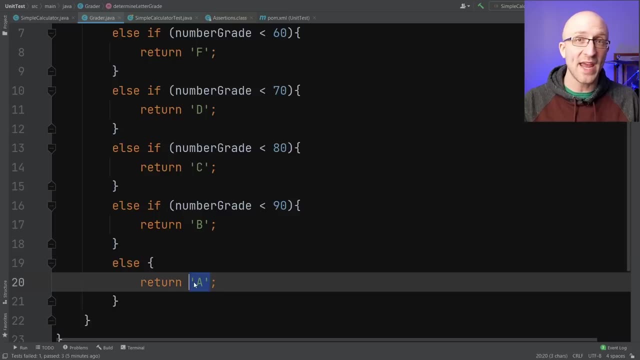 return an f for the grade. otherwise if it's less than 70, we return d. less than 80, we return c. less than 90, we return b. otherwise we know it's greater than or equal to 90. so we just return a First. we. 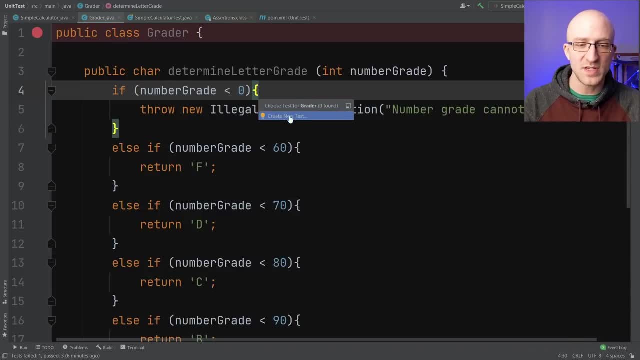 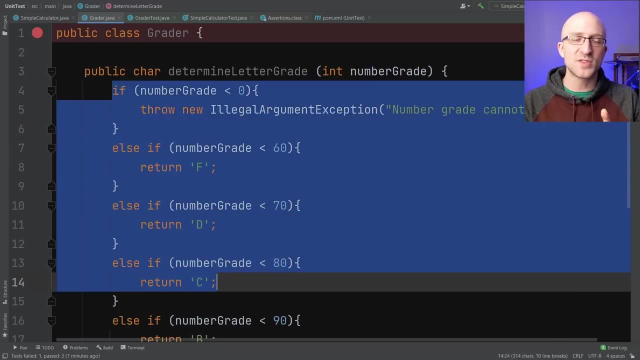 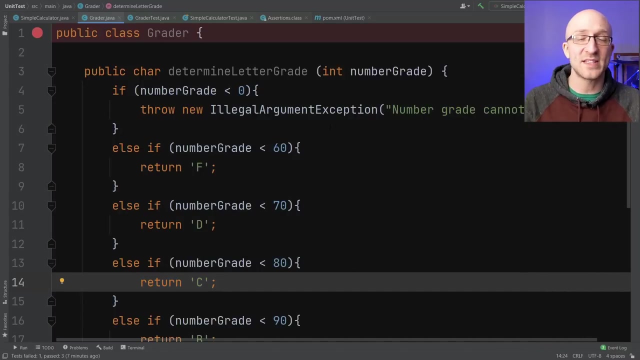 need to go ahead and create our unit test class. so we'll hit ctrl, shift, t as the shortcut and it's creating a class called greater test and let's hit okay. In this method we have a bunch of pretty simple test methods. Each separate scenario that we come up with should be tested in their own test. 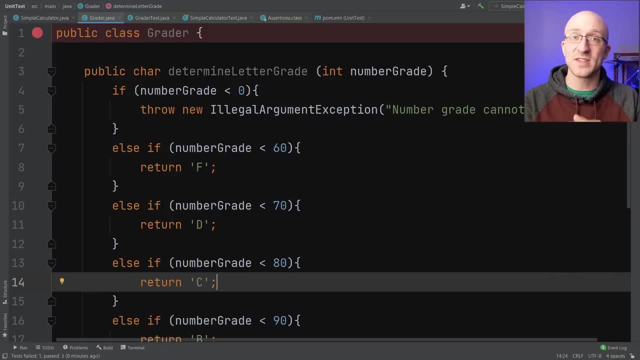 method. You should never combine multiple scenarios into one single test method. So, for example, one good scenario that we might want to test is that if we send in a 59 as the number grade, we should get an f as the letter grade. So let's go ahead and create that. Let's create a new test method. 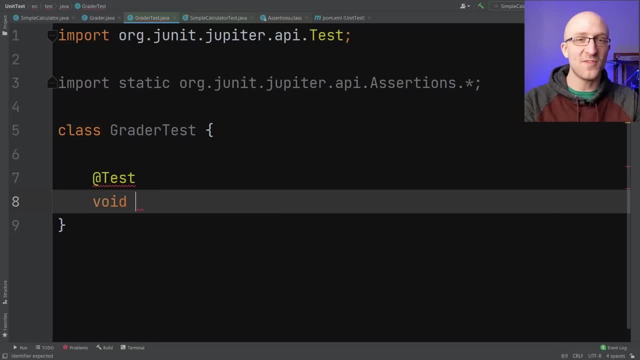 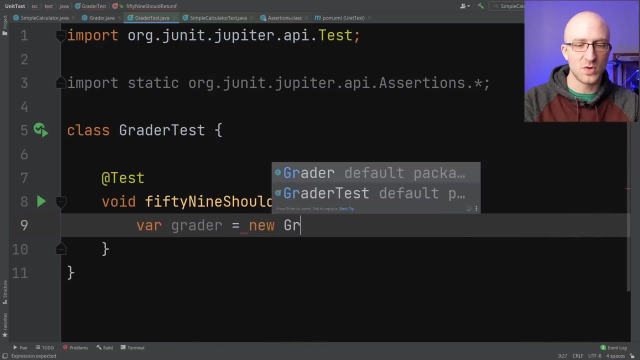 that we label with at test. Here we're just verifying that 59 should return f, so let's just say 59 should return f First. let's create our greater object so we can call that determine letter grade method on it: equals, new, greater, So similar to before. we want to assert that when we 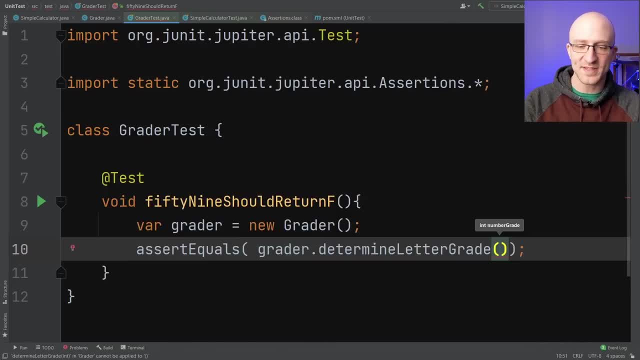 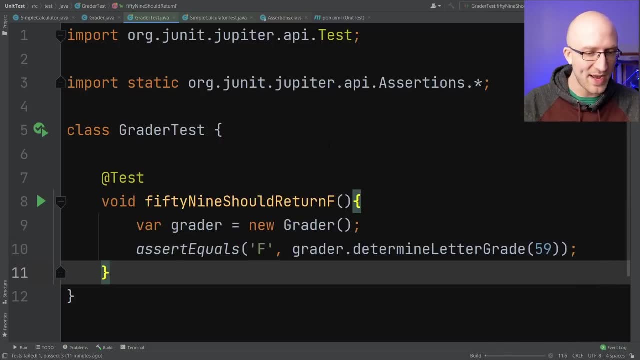 call greater dot, determine letter grade and pass in the value 59 that we get a result of f. Let's go ahead and run our test and make sure it passes- and it does Great. You may have noticed that over here, in addition to just running our test normally. 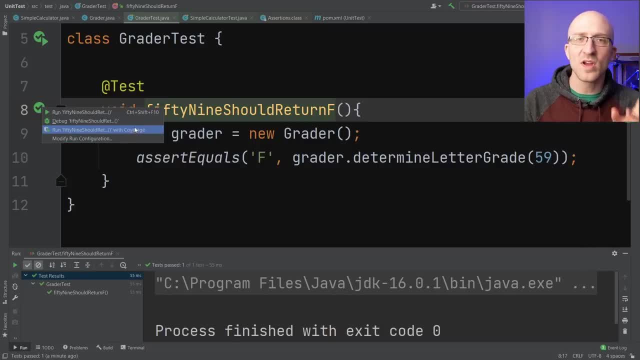 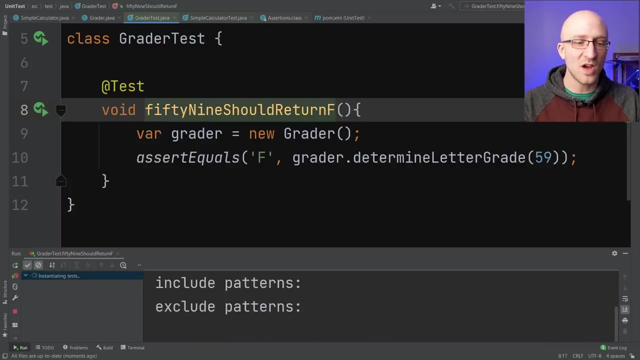 we also have an option to run our test with coverage. When we run our test with coverage, IntelliJ will show us exactly which lines of code were executed when our tests were run. So let's run this same test, but with coverage. Okay, so our tests run, they pass as normal. but then it also. 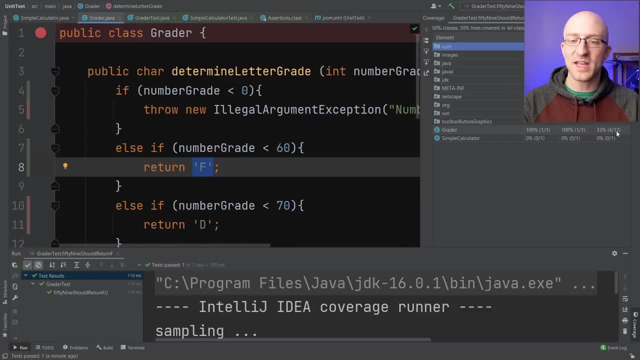 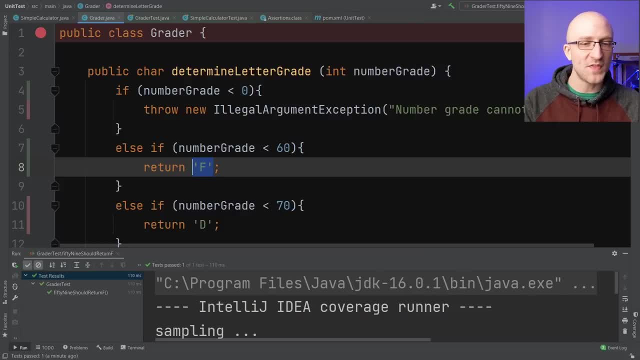 run this test and we're going to run this test and we're going to run this test, Then that will expose the error. We can see here how it flies out of the chronology function of our test. So we can see that it's showing that we're hitting three out of 12 lines in that class, four out of. 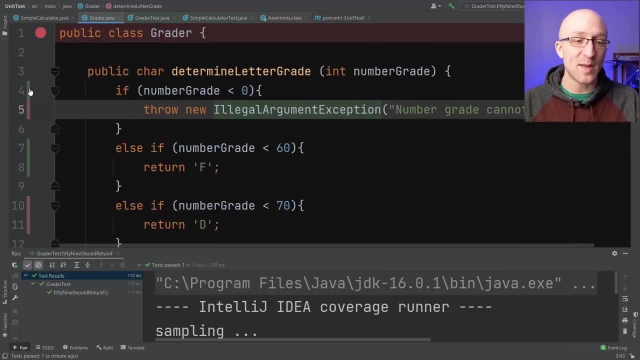 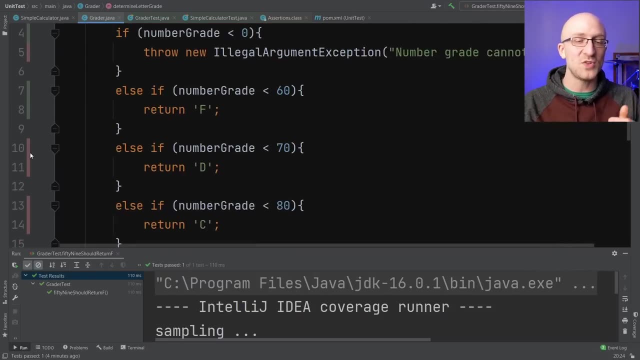 12 lines and if we look over here at the actual class in the editor Here, you'll see different colors- green or red- depending on whether the unit test that we just ran hit that particular line or not. One of our goals for the unit test that we write for this method should be that we eventually 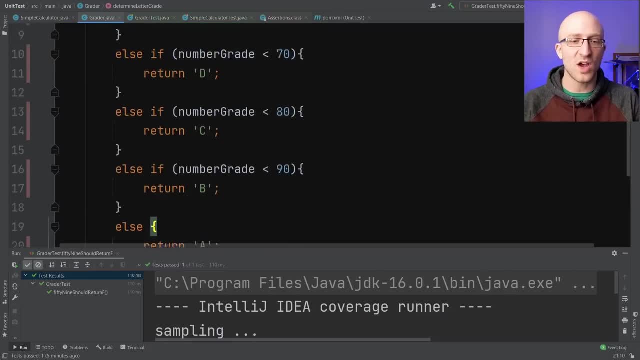 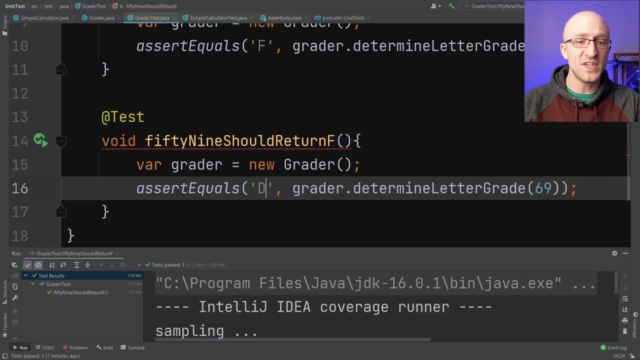 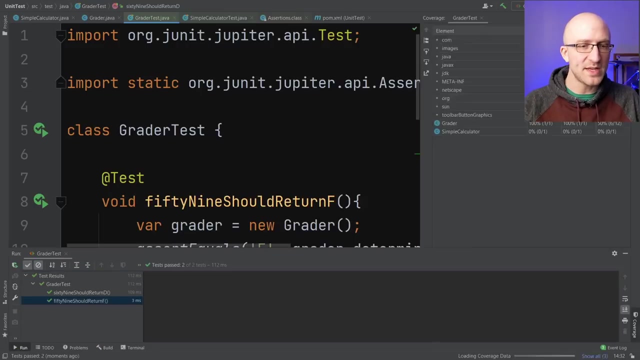 that let's write more tests to cover each of these other scenarios. so maybe another good test would be that a 69 should return a letter. grade of d 69 should return d run greater test with coverage. okay, it's complete, our tests pass. now let's look at the coverage over in greater test and it shows. 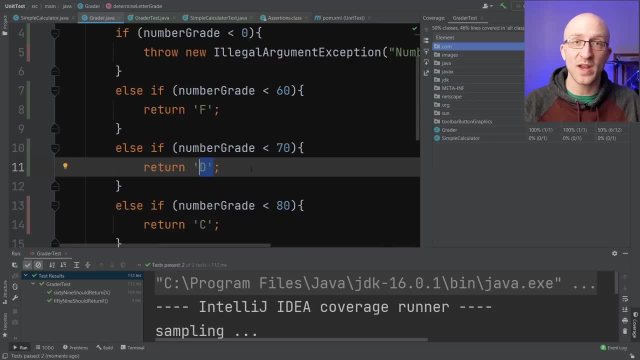 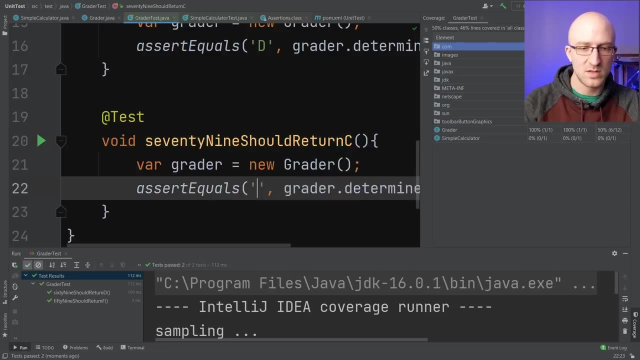 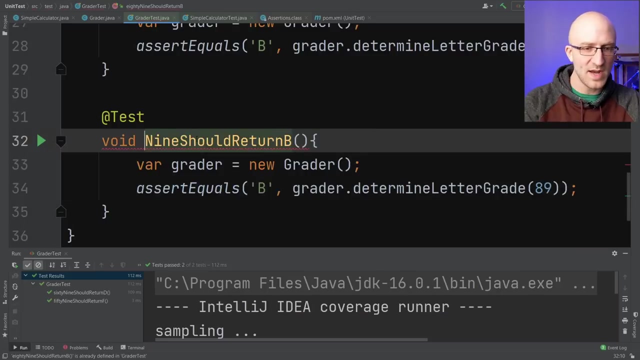 that. yes, we are now hitting lines 10 and 11 because they're showing as green, so let's go ahead and do the same thing for c, b and a. 79 should return c, c, 79, 89 should return b, b, 89, 99. 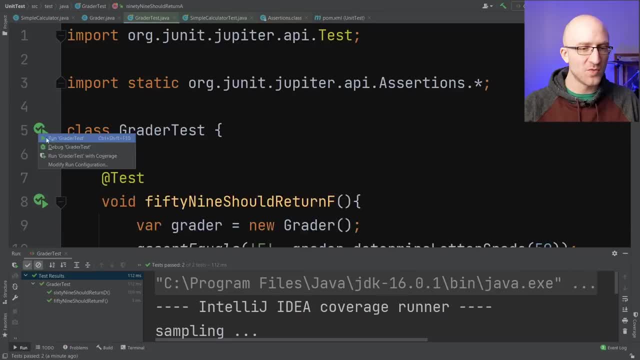 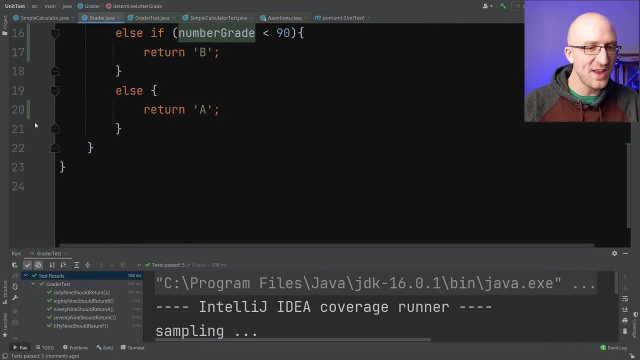 should return a, a, 99. run greater test again with coverage and it's looking good. all of these situations- f, d, c, b and a are all green now because we're hitting all of those scenarios. the only line left where it says c, b and a are all green now because we're hitting all of those scenarios. the only line left where it's 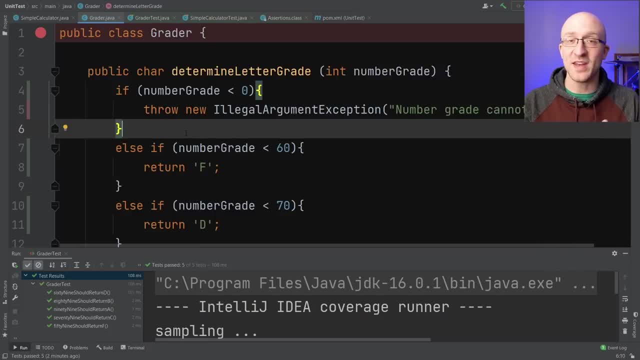 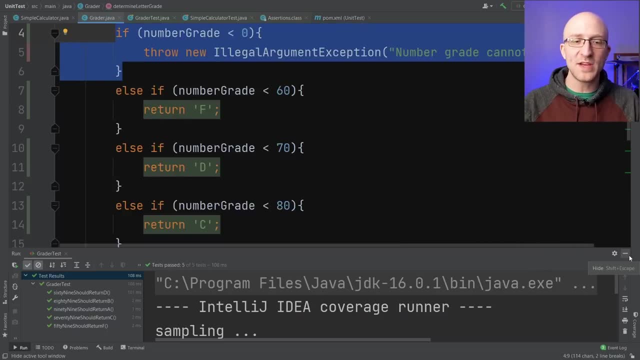 still showing red is line five here, where when we send in a negative number, it throws an exception. we'll talk more about how to handle this exception scenario in just a moment. first, we want to make sure that our tests are handling all of the possible edge cases in all of these simple 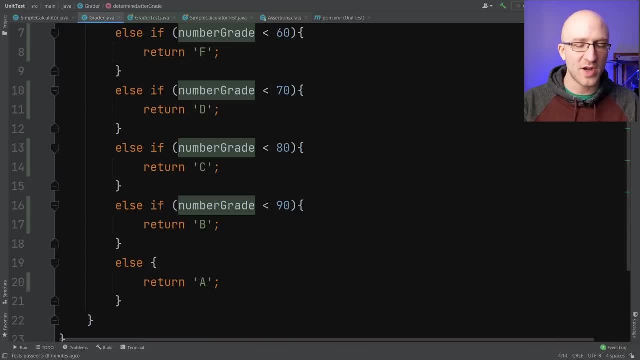 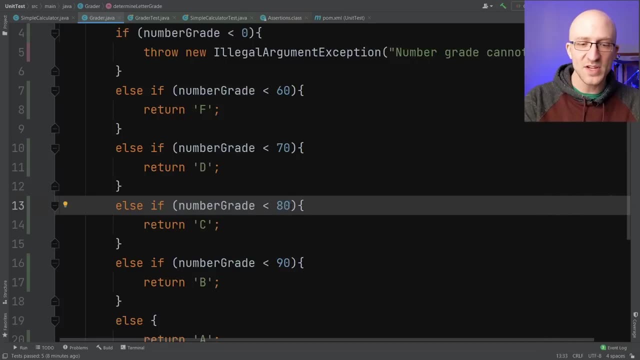 scenarios. let's say i went over into our determined letter grade method and changed the criteria for getting a letter grade of c to being, instead of less than 80, i changed it to less than 81.. right now if you pass in a number grade of 80, it will hit this condition and return the value of c. 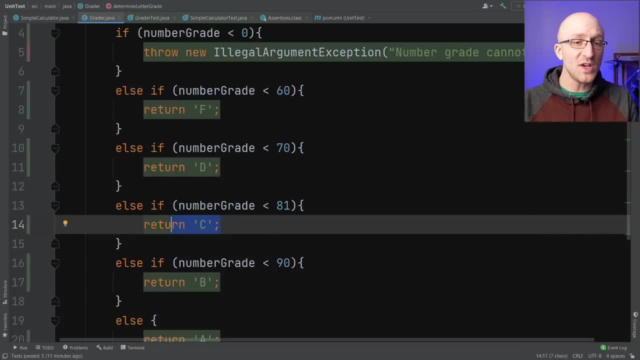 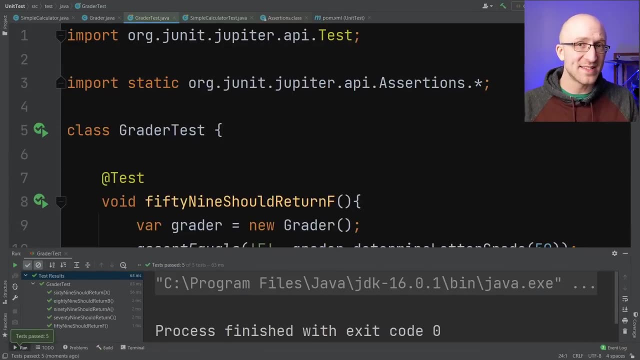 when an 80 should be a b instead. so we have a situation where our code is wrong. but if we go back and run all of our unit tests, they all pass and say that everything is okay again. this doesn't necessarily mean that our test scenarios are bad, it just probably means. 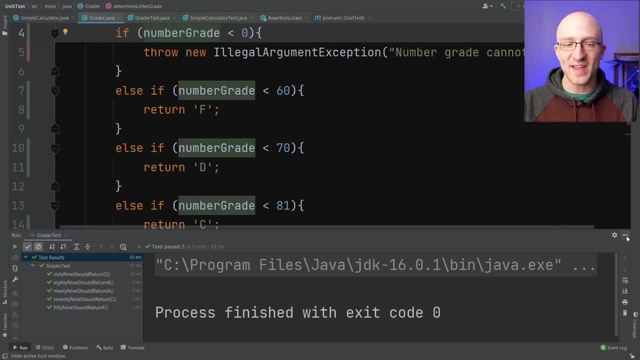 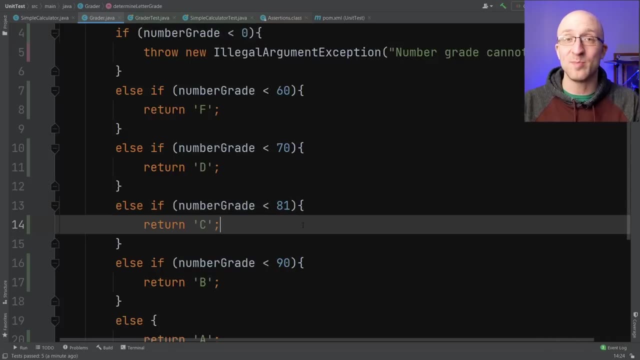 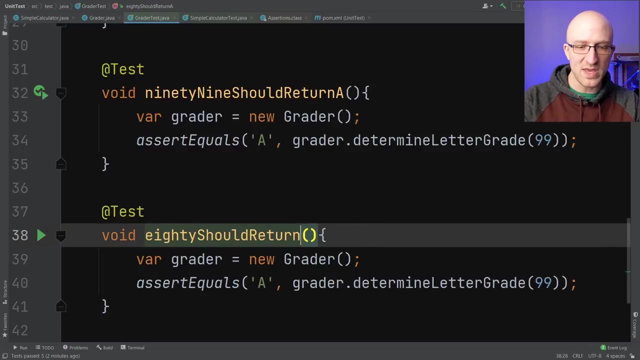 that we need more of them. so, for example, we should have a test scenario that validates that edge case where if we pass in an 80, it returns a, b, as it should. so let's go ahead and create that test case. so 80 should return b. so if we send in a letter grade of 80, it should return. 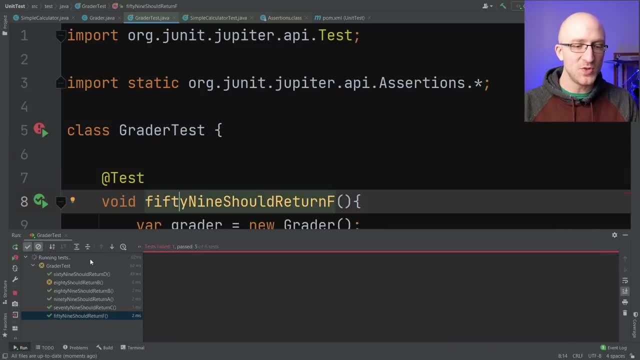 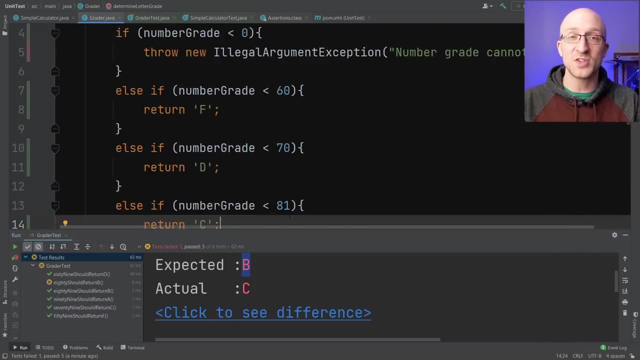 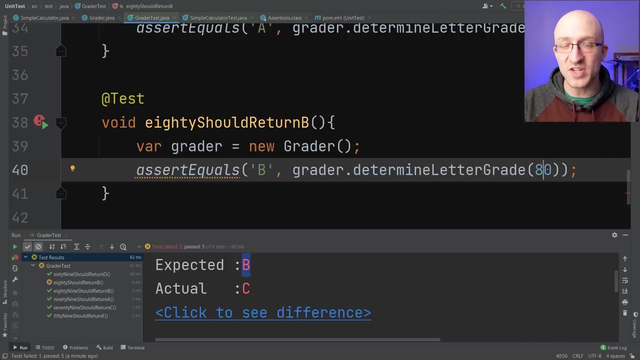 b, let's rerun all of our tests. and now we do get one failing test, and this test failure is good. our code is currently wrong, it's not doing what it should do, and so we should have at least one failing test. and now we have a test scenario to cover that edge case: that an 80 should return a b. so now, 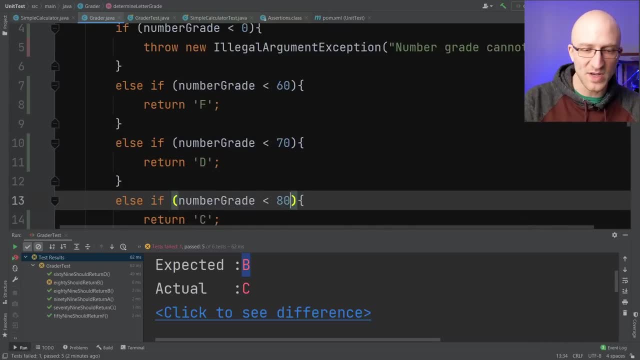 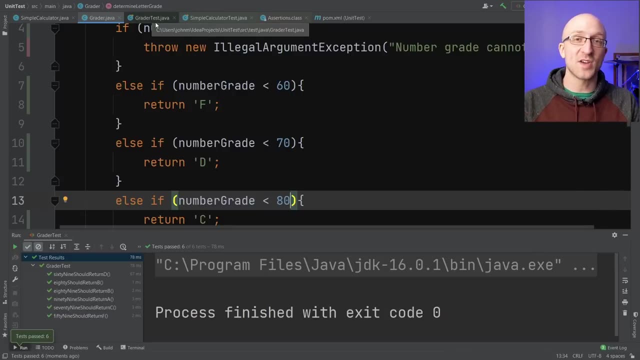 if we go back and fix our code to change this back to an 80 and rerun our tests and they all pass. but now, with that added scenario, our unit tests are that much stronger and more strictly guarantee that our code is doing exactly what it should. so let's go back into our tests. 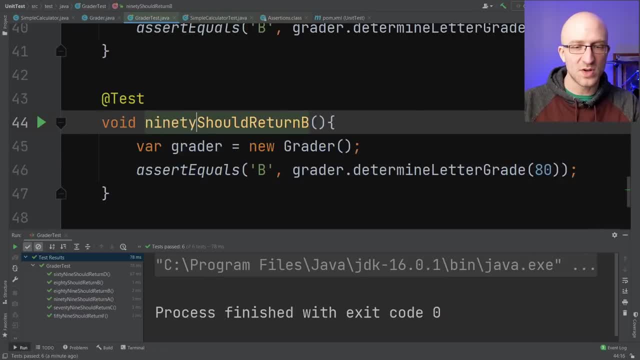 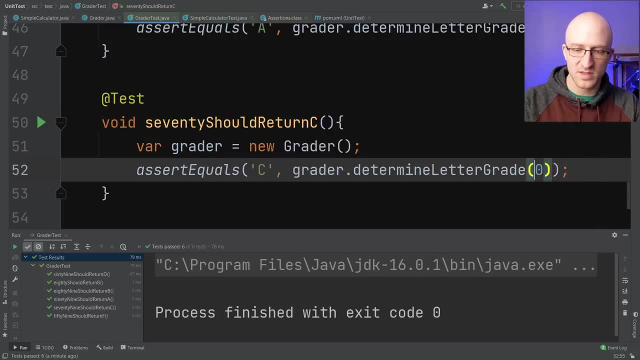 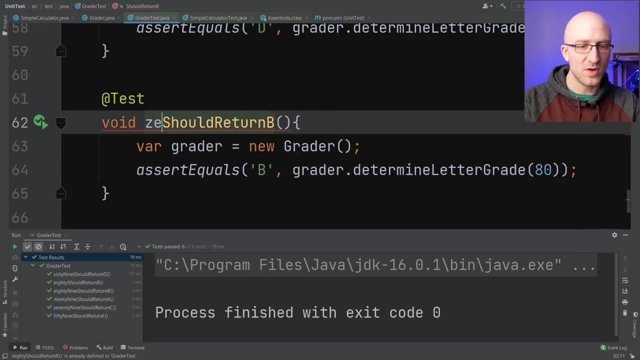 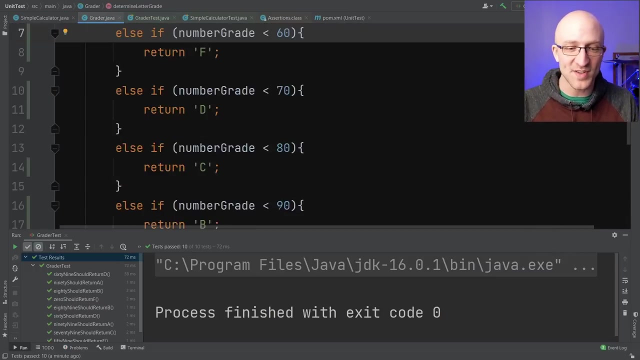 and add some other edge cases: a 90 should return a, a 90, 70 should return c, c, 70, 60 should return d, d, 60.. finally, zero should return f, f and zero. okay, so they all pass. but now our unit tests are even stronger than they were before, so we can go in. 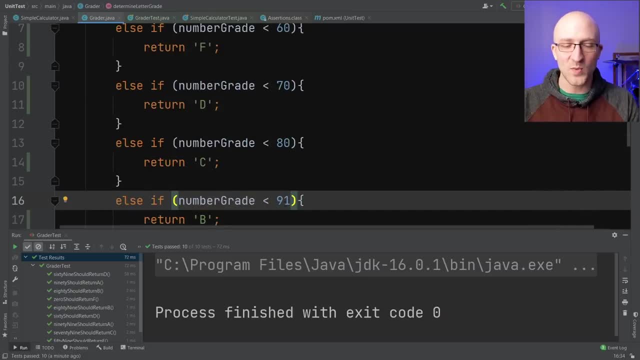 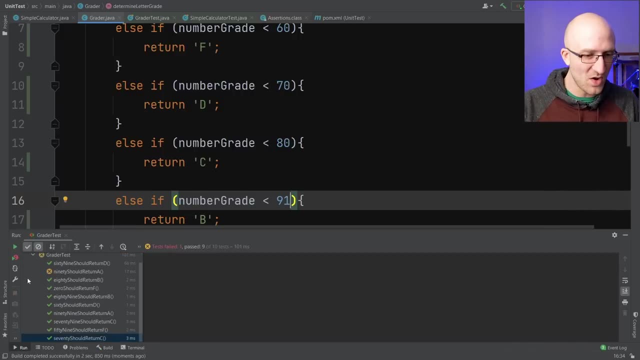 and mess around with any one of these numbers and just change it by one. like we can change this 90 to a 91 and run all our unit tests again and a least one of them is going to fail. so here we go and 90 should return. a is failing because now. 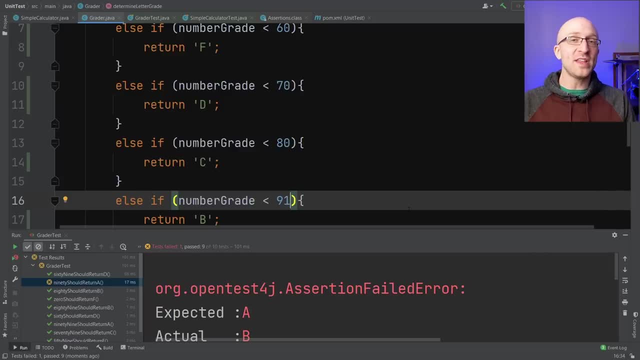 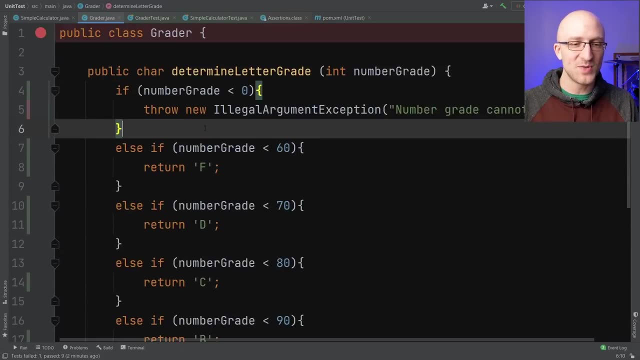 a, 90 is returning b, so that's really great. we have a really strict set of unit tests that are guaranteeing the proper functionality of our code. okay, so let's get back to this scenario here, where if you send in a negative number, it throws an illegal argument exception. so in our 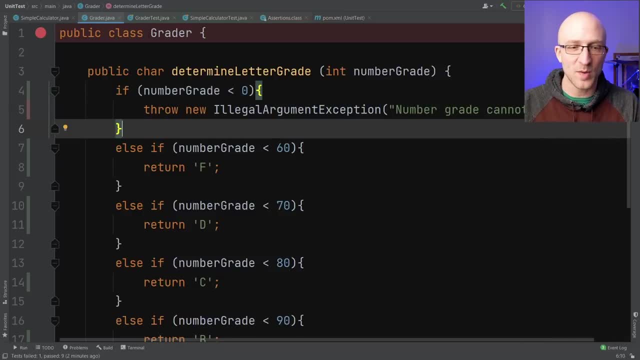 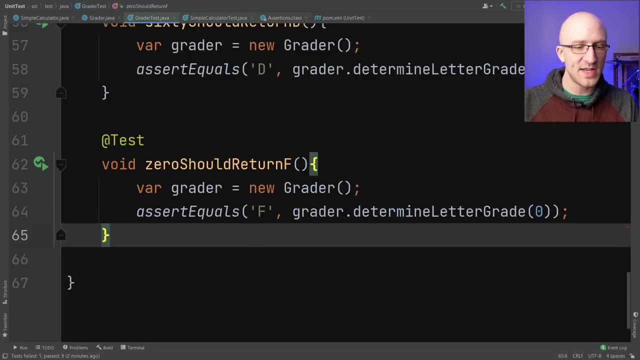 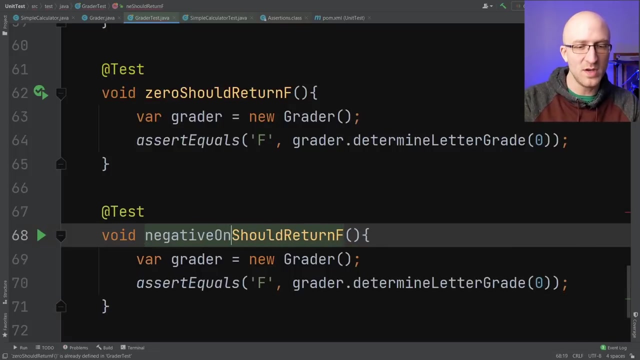 unit test. we do want to have a scenario where, if we send a negative number, we verify that it's throwing an exception, as it should. but how do we do that? so first let's hop back over to our test class and, uh, just try it out. so let's go ahead and copy this test method and we can say: negative, one should return. 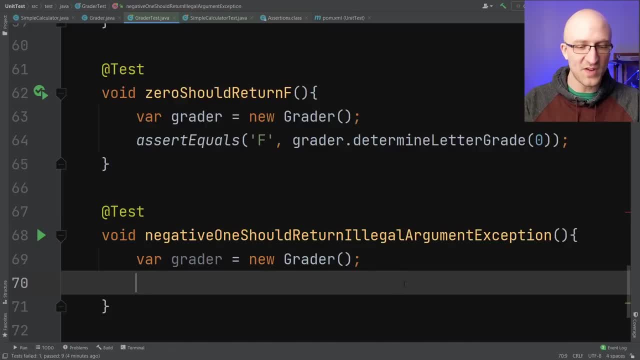 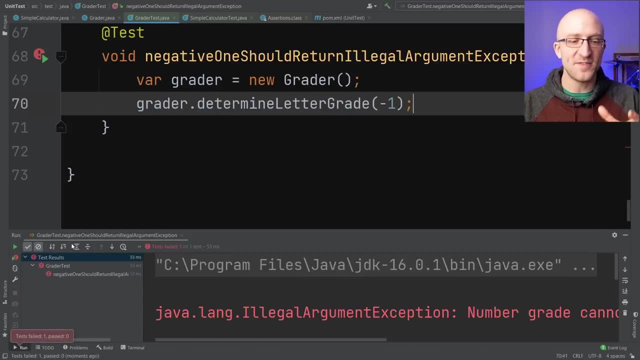 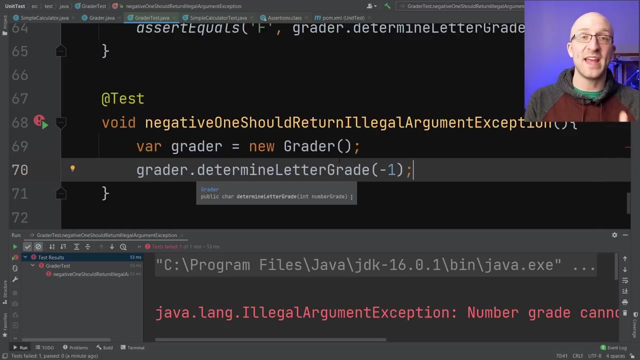 illegal argument exception. and let's just verify what happens if we call this: determine letter grade method with a negative number and right now the test fails. under normal circumstances, if the code that you hit throws an exception, it will automatically fail your unit test. instead, there's a certain assert statement that you can use in j, unit 5 that asserts that an 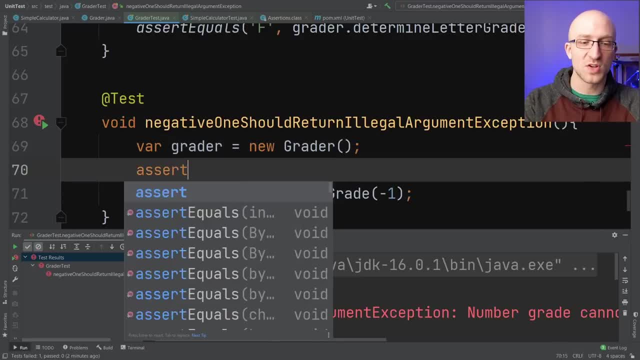 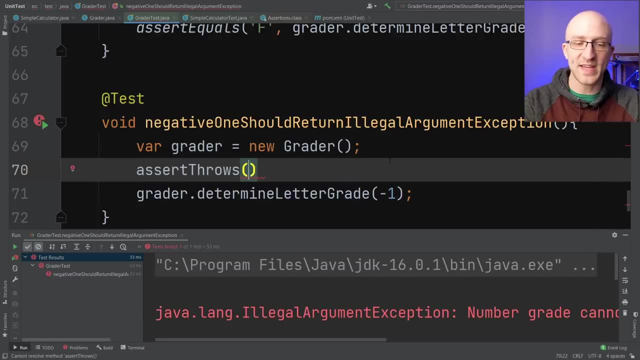 exception was thrown and that assert is called assert throws. now this assert throw method also takes a couple of parameters, but it works a little bit differently. the first parameter that it takes is the name of the class of the exception that you expect to be thrown. so here we expect an illegal. 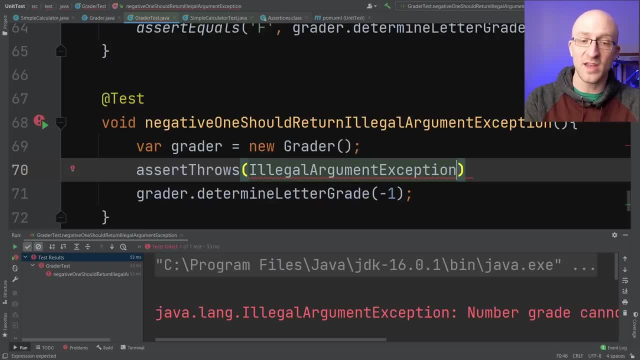 argument exception to be thrown. so our first parameter is going to be illegal argument exception. the second argument that it takes is actually the executable piece of code that you need to call to get that exception to be thrown. you can do that by using what's called a lambda- now lambdas. 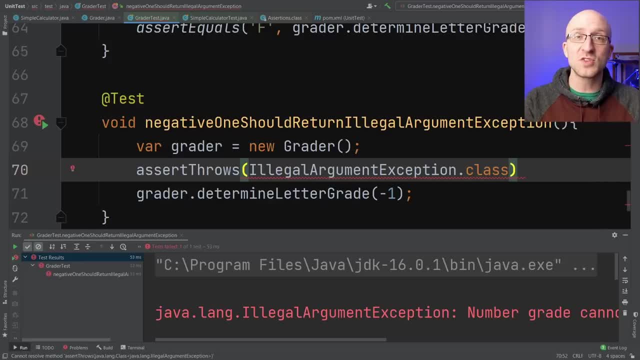 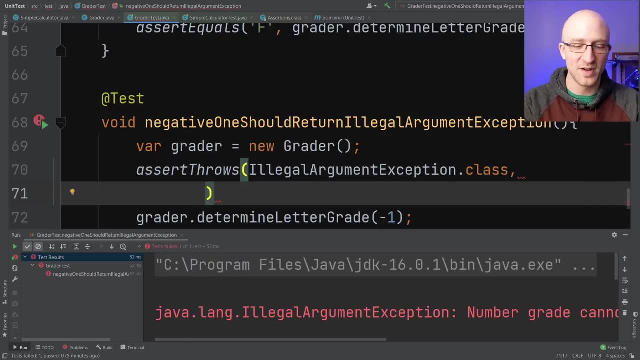 themselves are a whole other topic, for an entire other video. so i'll just show you what you need to know to get them to work for this particular use case. so to pass in your lambda as your second parameter, you would first just do an open and close parentheses, then space, hyphen and greater. 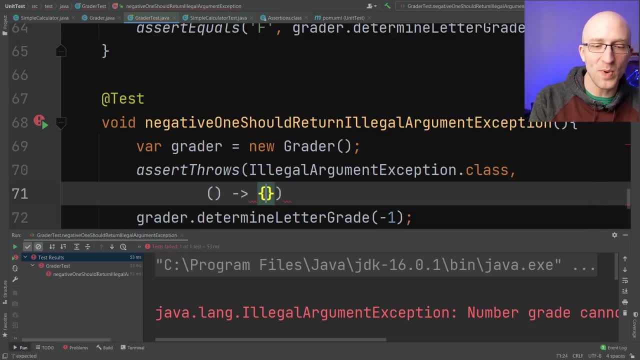 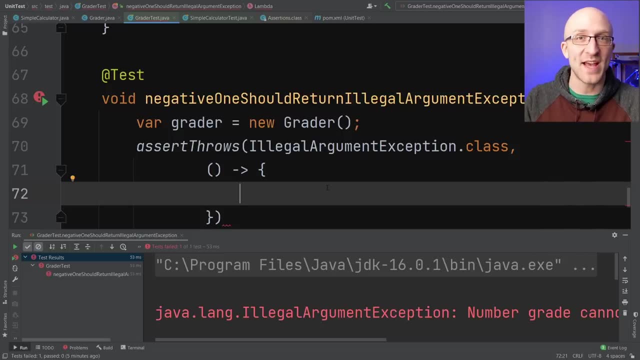 than so. it kind of acts like an arrow, and then you want to open a curly braces and then inside those curly braces is where you want to put the code that executes your test. so in our case, the code that we want to run, that will make this. 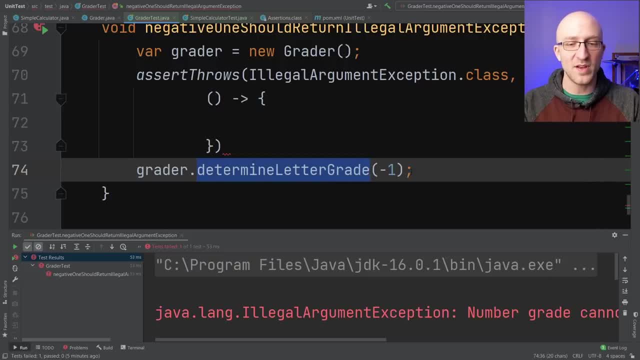 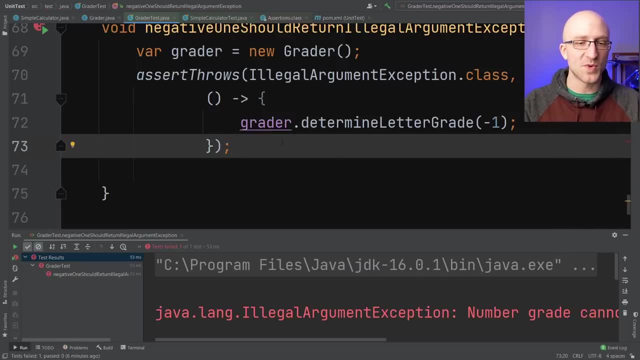 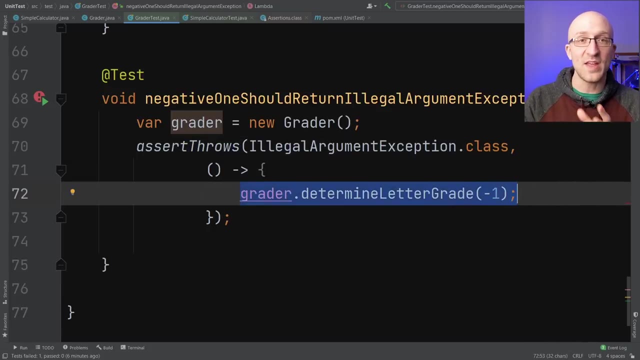 exception get thrown is calling this determined letter grade method with a negative one as the parameter. so we'll just paste that on in here and put our semicolon here after the close parentheses. so what this assert throws is doing is it's verifying that when this piece of code is executed, 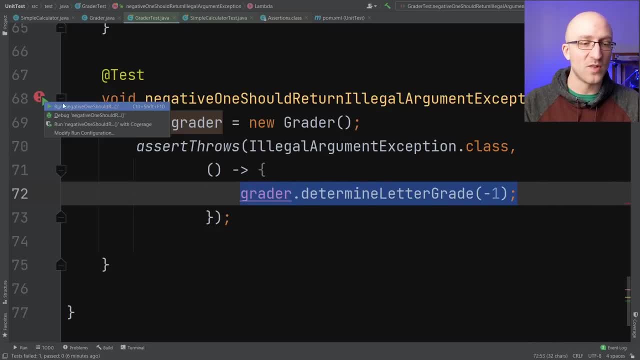 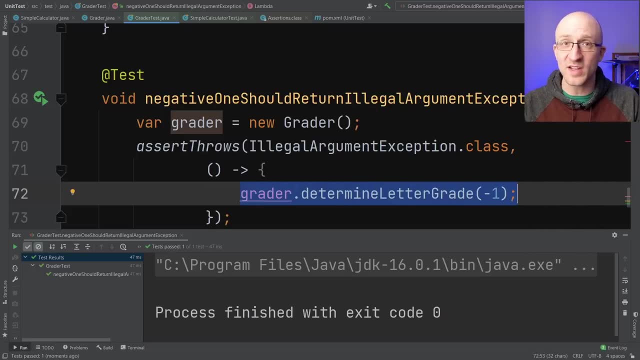 it throws a small number. so return home, for a set number of decimal places in ep, root of in geral, an illegal argument exception. So let's go ahead and run our test and make sure it passes And it does. If calling this piece of code wouldn't have thrown an illegal argument exception, then our test. 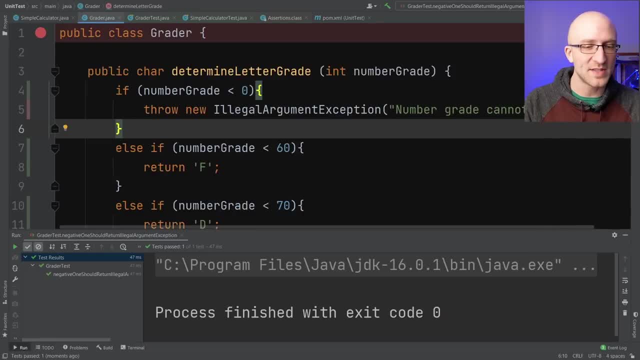 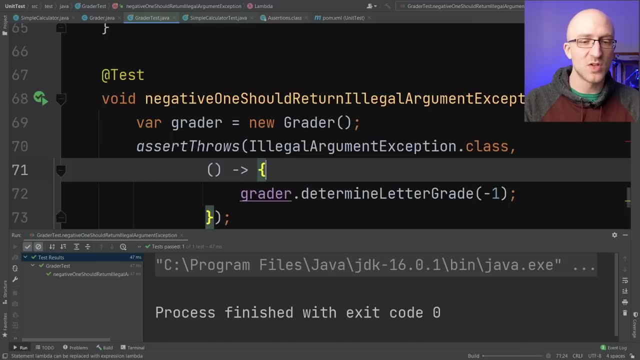 would have failed. So, for example, we could go back into our grader class here. So what if it didn't throw an exception and instead returned a letter grade of f? So when we run our test, we would expect this to fail. And that's exactly what it does. It says we expected an illegal argument. exception to 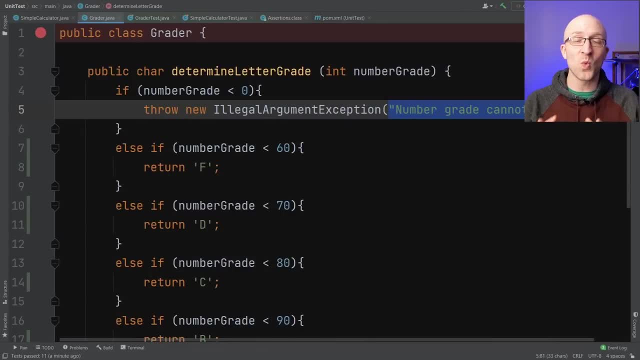 be thrown, but nothing was thrown. So that leads us to the reasons why it's a good idea to write unit tests for your code. First and foremost is the obvious reason: It ensures that your code is actually correct. You don't have to be pretty sure that your code is correct. You can write a bunch. 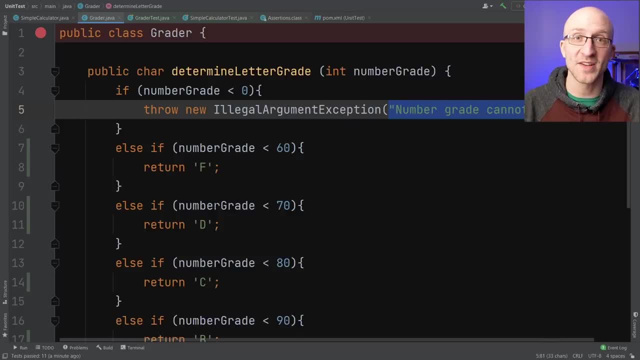 of test scenarios to be absolutely sure that your code is correct, And I even often find myself making changes and improvements to code as I'm thinking up new unit test scenarios. So it makes my code better when I write unit tests. Once you have a comprehensive suite of unit tests in place that guarantee that your code is working. 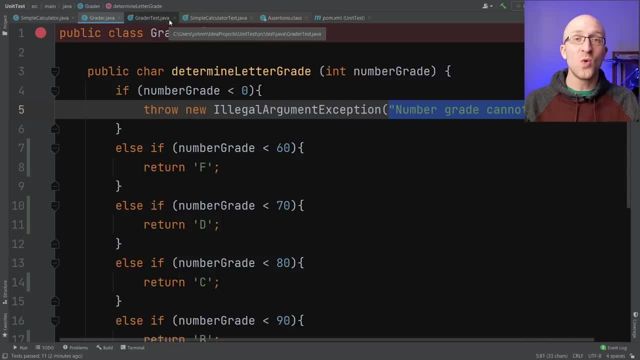 the way that it should. you can refactor that code any way you want, with absolute confidence, Because you know that if you refactor it in such a way that you mess up the code a little bit, one of your tests is going to fail and tell you that there's something that you need to fix. So for 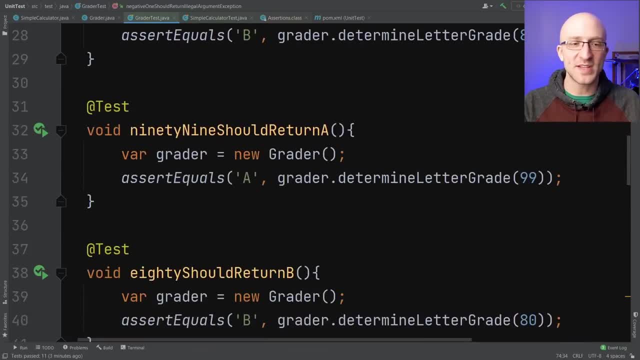 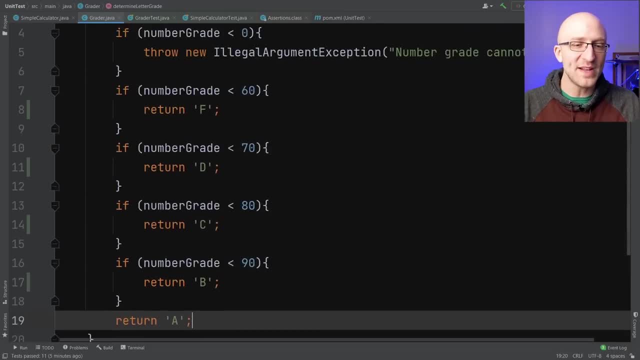 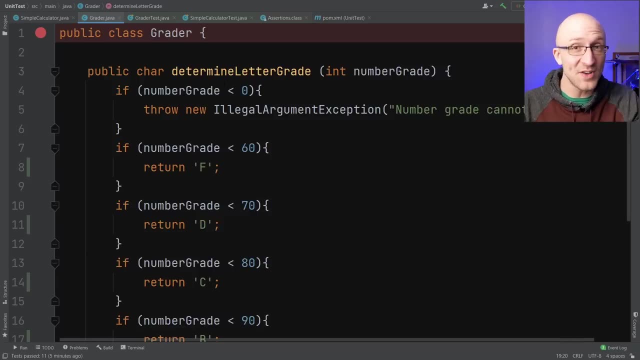 we can refactor in such a way that we can refactor in such a way that we can refactor in such a way that rid of that one, that one. so now we've made some changes into this class that might scare you if you don't have a complete set of unit tests ready to hit your code really hard and make sure that. 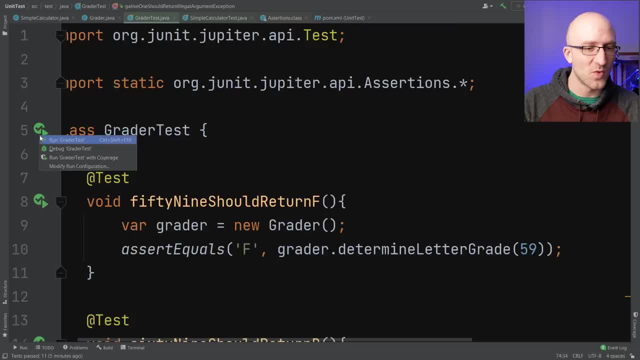 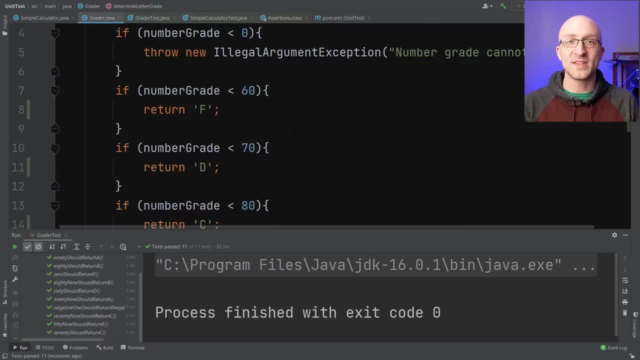 it's doing what it should, so we can go back to our greater test and run all of them again, and here they go, they all pass, and so we know that, even with the changes that we made, our code is still doing exactly the right thing. the subject of unit testing is a really, really deep one, and 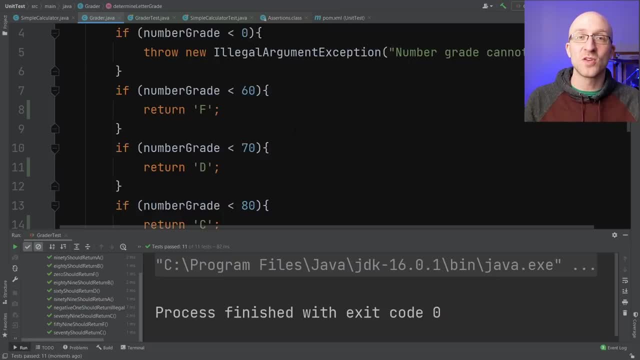 we've just scratched the surface here. as always, if you enjoyed this video or learned something, please let me know by leaving a like and hit the subscribe button, so you don't miss each new java tutorial. and don't stop here. keep up your learning momentum by checking out one of the other videos. 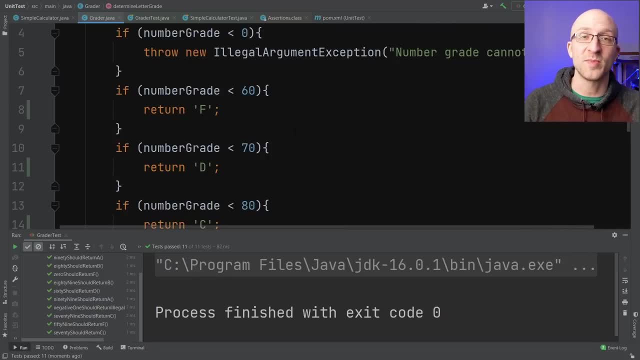 below. thank you so much for watching. i really do appreciate you being here with me. i'll see you next time. 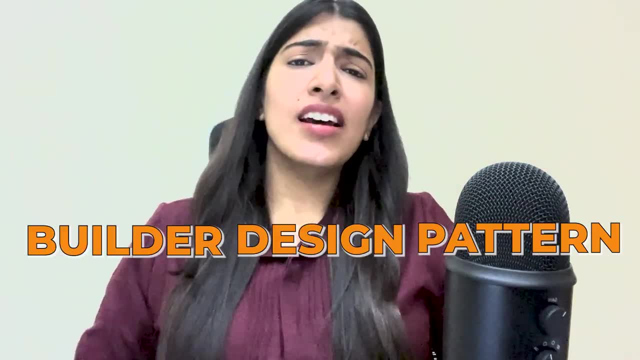 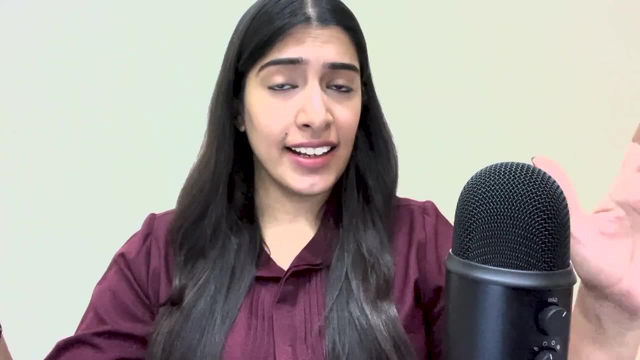 Hi guys, today we will be discussing build a design pattern. Now, this is one of those design patterns that I personally took a lot of time to understand. We are going to break it down to very simple parts and understand. Okay, it is a creational design pattern, as